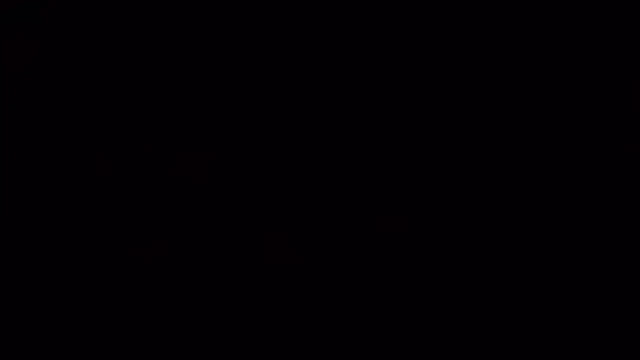 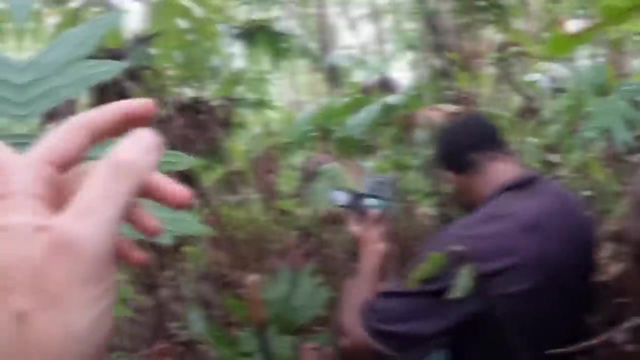 felt like finding a unicorn, said John Mittermeier, who helped lead the expedition. It's the kind of moment you dream about your entire life as a conservationist and birdwatcher. Even though there aren't many records, the Conservancy says it's likely that the number 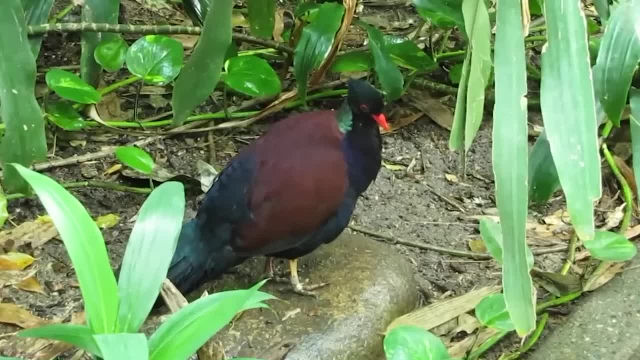 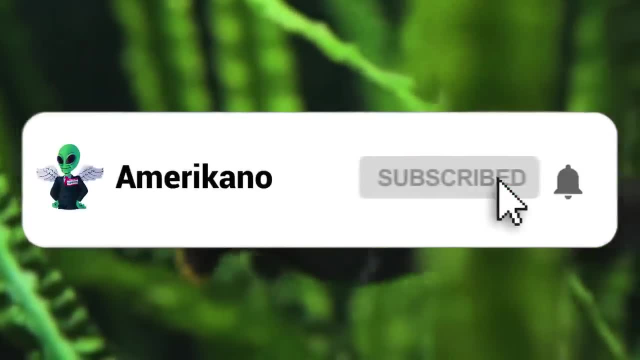 of ground pigeons on the island is small and declining, So it could be a long time before we see it again, if ever at all. Before we go on like this video, smash that subscribe button and click the notification bell right now, or the centipede will crawl on your face when you're sleeping. 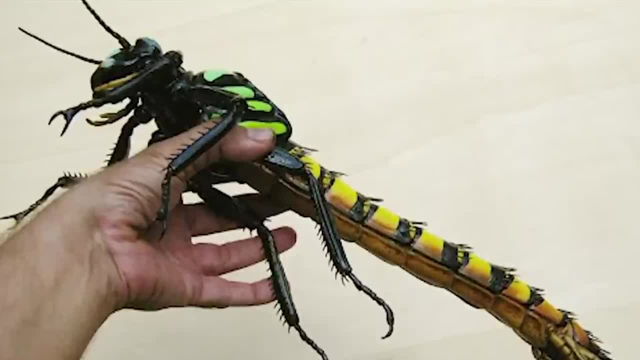 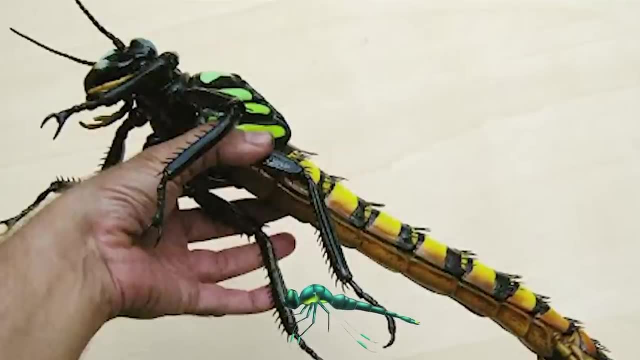 Time for the rare topic. Back in the 19th century, some paleontologists amazed the world when they produced a fossil they had dug up that showed the outline of an absolutely huge dragonfly. This was, in fact, terrifying, and pretty much everyone in the Victorian era agreed that they were lucky. 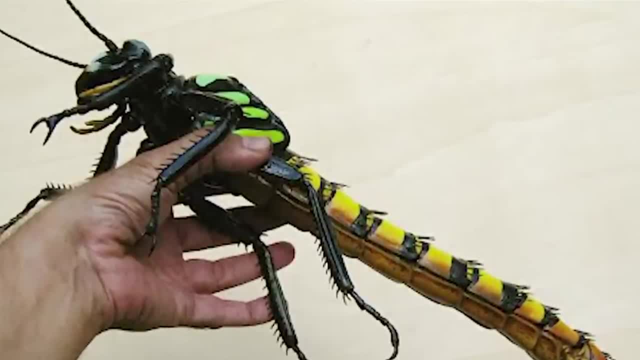 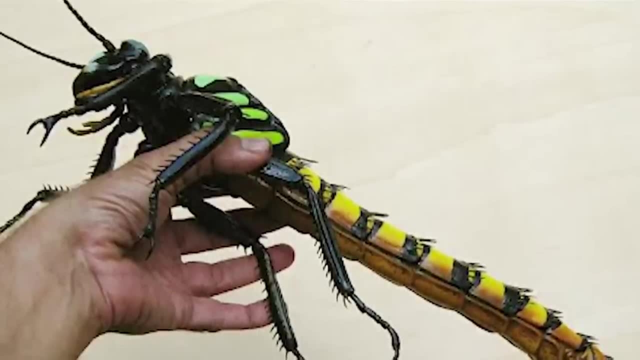 not to live on a planet with a thing like that flying around. Fast forward to 2023, and a new generation of scientists have got some bad news. This monster insect isn't extinct at all. In a scene that could come right out of a Hollywood movie, a giant dragonfly appeared in a 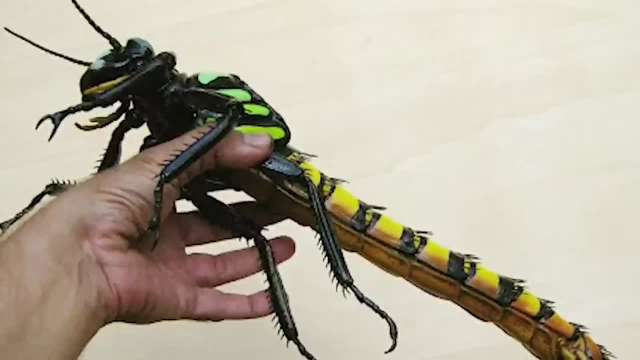 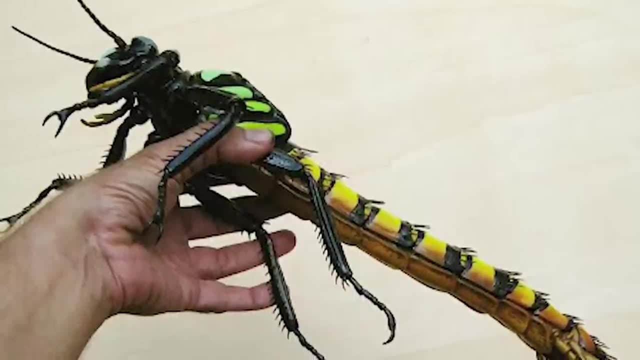 camp for researchers in Borneo and let them know that it was very much alive. Some claimed it was even breathing fire. Uh, that might have been just some panic and strong imagination, But if you're curious, what do you think about this dragonfly? Should we just leave it alone? 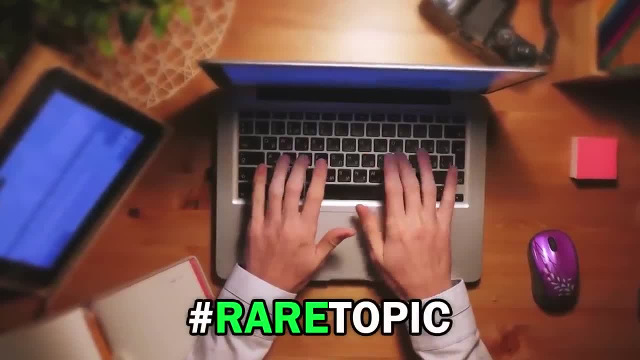 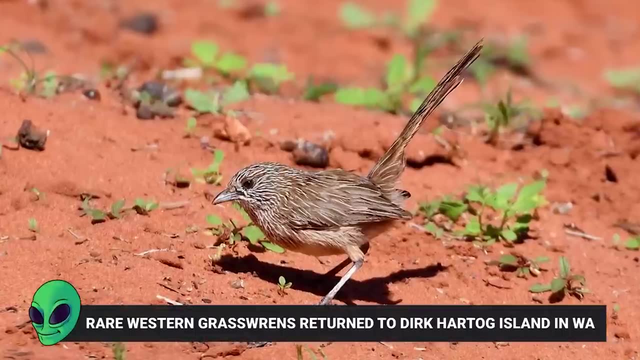 As always, comment down below with the hashtag Rare Topic and let us know your opinion in relation to what we just showed on screen. Let's move on to the next one: 19. Western Grass Wrens Return to Dirk Hartog Island in Western Australia. 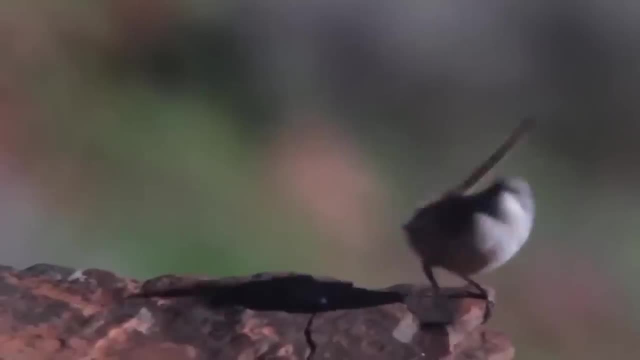 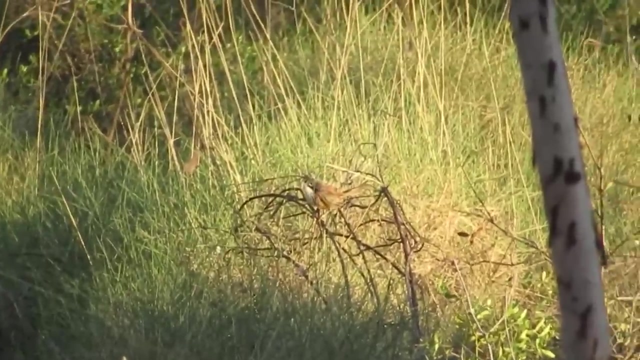 On Dirk Hartog Island in Western Australia, the call of the Western Grass Wren can be heard again for the first time in 100 years. The rare story is that the Western Grass Wren, which is the largest species, was just moved to the island which the Malgana people called Wiriwana along. 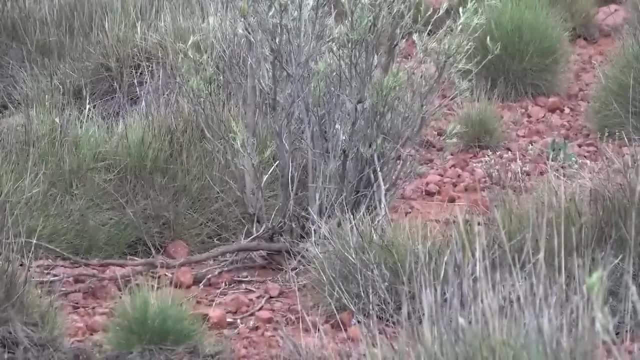 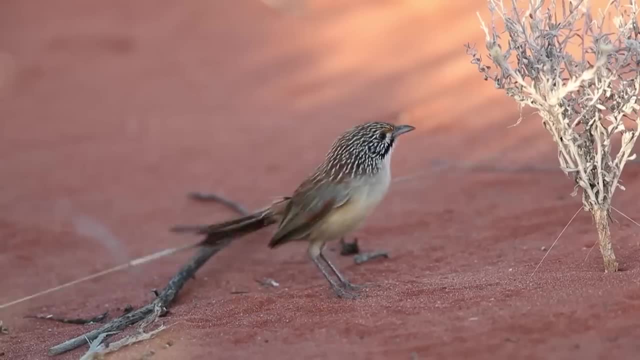 with wrens from the two different parts of Shark Bay. At first, many people wondered if the two birds from two different groups would understand each other as they trill in different ways. Birds call for many different reasons, but the Grass Wren's territorial song is very important. 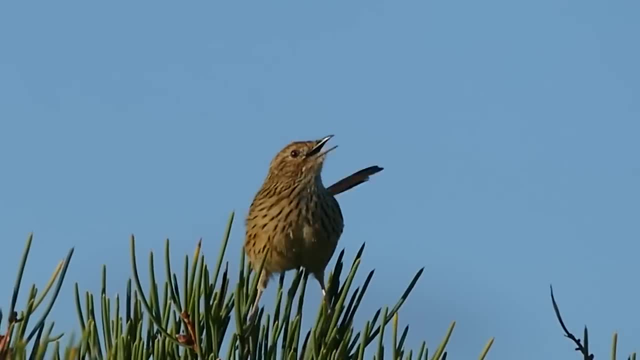 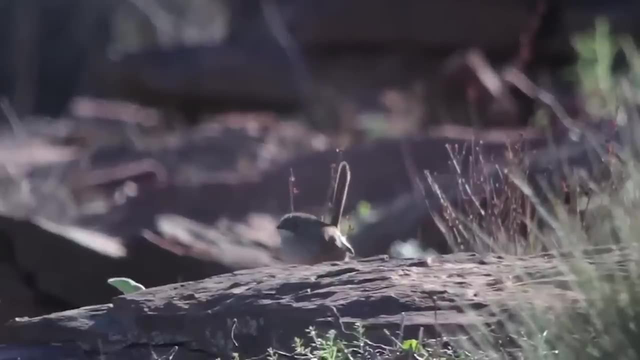 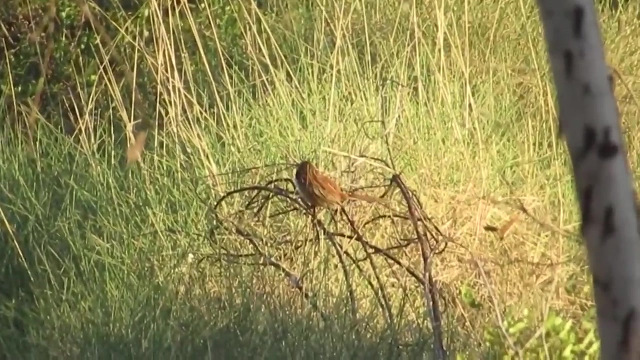 20. French and Spanish. So it's kind of like these two groups of birds are speaking French and Spanish. They might understand each other at times, but they might also not. Thankfully, even though the territorial calls were different, they weren't different enough to cause any dialect. 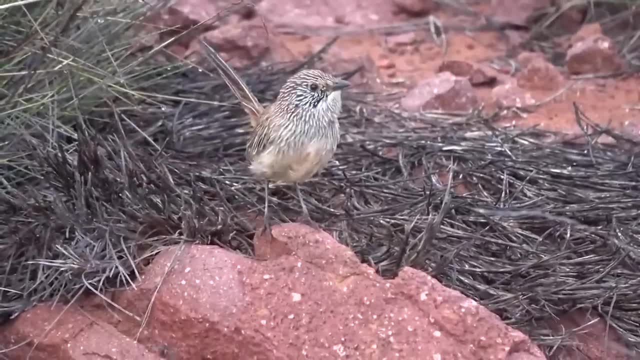 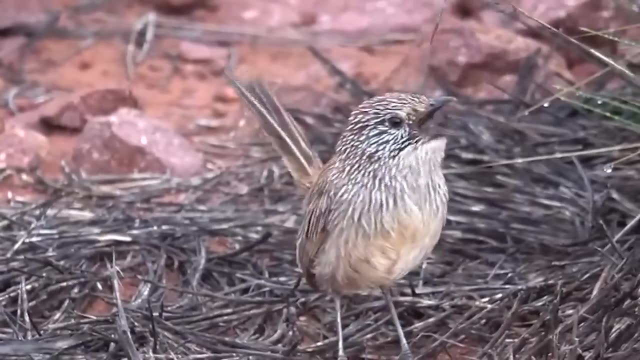 problems. The wrens are one of 13 species that are being brought back to Dirk Hartog Island as a part of one of the biggest projects of its kind. Putting the birds on the island will also help protect the future of the species. This is all part of the Return to 1616 Ecological Restoration. 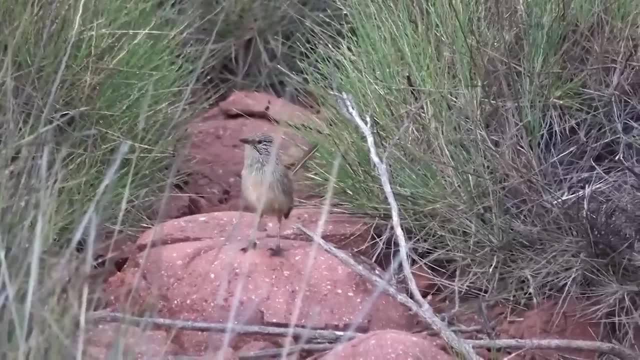 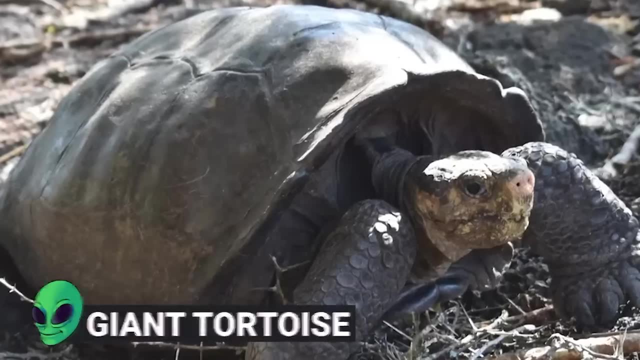 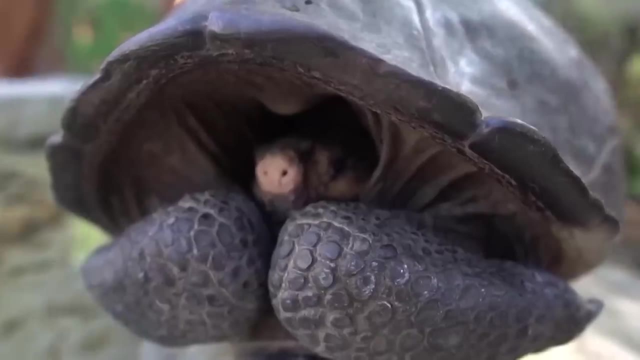 Project which aims to make the island look like it did when the Dutch explorer, Dirk Hartog first arrived more than 400 years ago. 18. Giant Tortoise: Scientists have confirmed that, a rare species of giant tortoise that had been thought to be. 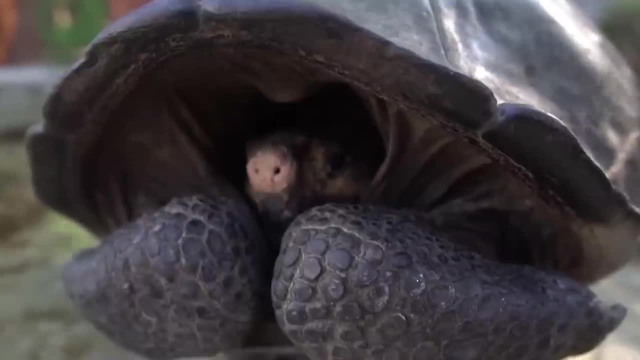 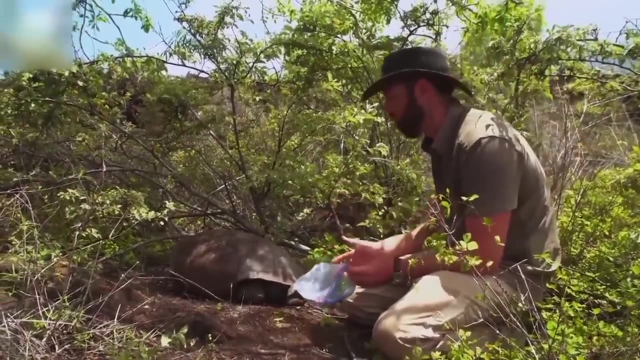 extinct for more than 100 years, is still alive in the Galapagos. Welcome back, slow-moving friend. A single female tortoise was found on Fernadina Island in 2019.. They named her Fernanda, which isn't super original. We can be honest about that. When Fernanda was born, she was a small. 5-foot-tall tortoise. She was born in the Galapagos and was born at the age of 17.. When she was 12, she was born in the Galapagos and was born in the Galapagos. and was born in the Galapagos and was born in the Galapagos. 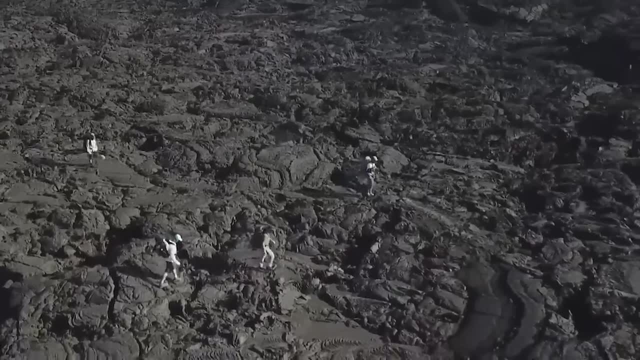 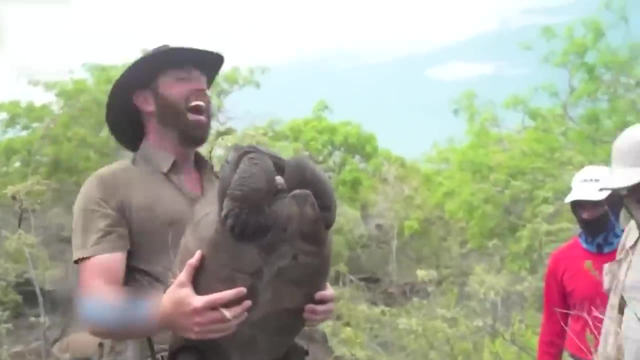 in the Galapagos. When Fernanda was found in 2019, roaming in a clump of plants among the hardened lava of the islet, it gave researchers hope that the rare Phantasticus species wasn't extinct after all. And yes, Phantasticus means fantastic. This is known as the fantastic giant. 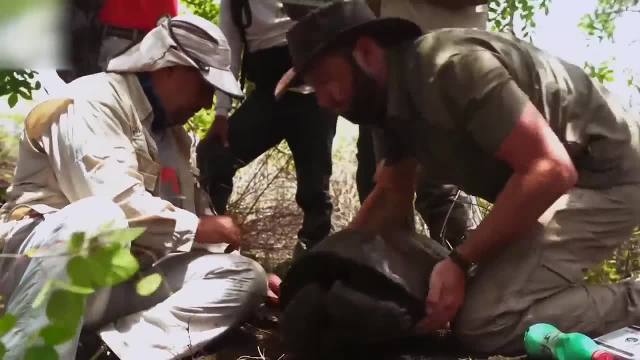 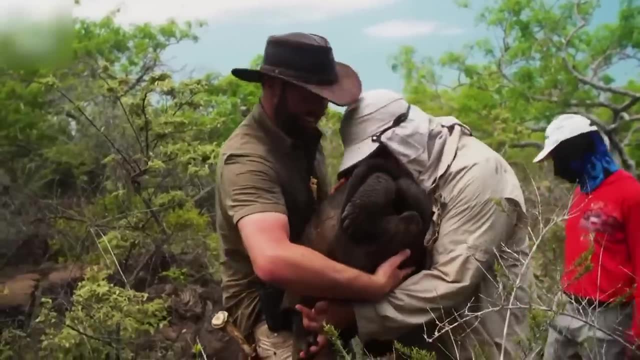 tortoise. However, they had to test Fernanda's DNA to confirm that their hopes were true. Fernanda is probably at least 50 years old, but she's smaller than most giant tortoises. This is likely because there wasn't much vegetation on the dry. 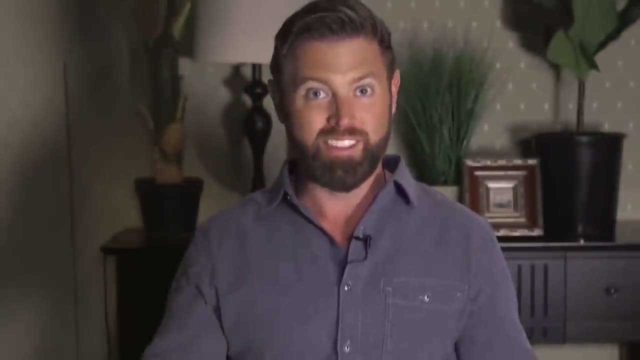 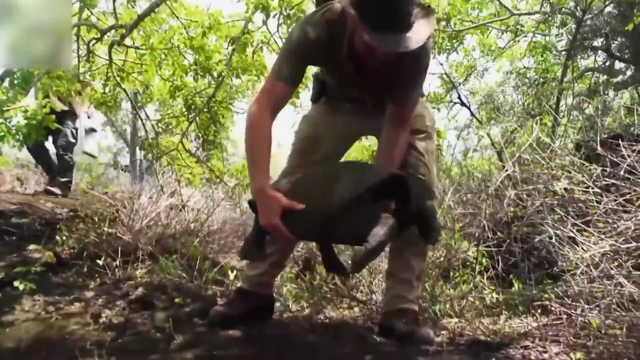 volcanic island where she lives. This was one of the reasons why scientists at first didn't think Fernanda was a native Fantastica species. The other reason was that Fernanda didn't have the flared shell and saddleback shape of Fantastica. The fantastic giant tortoise hadn't been seen. 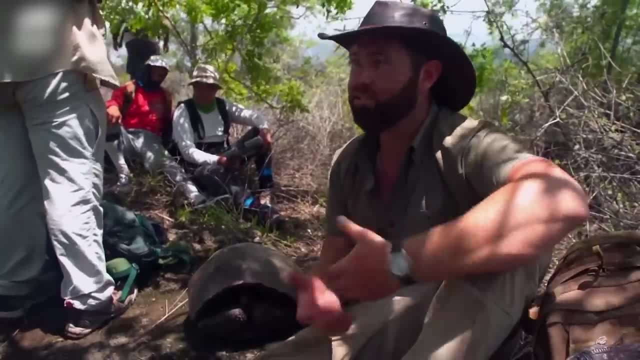 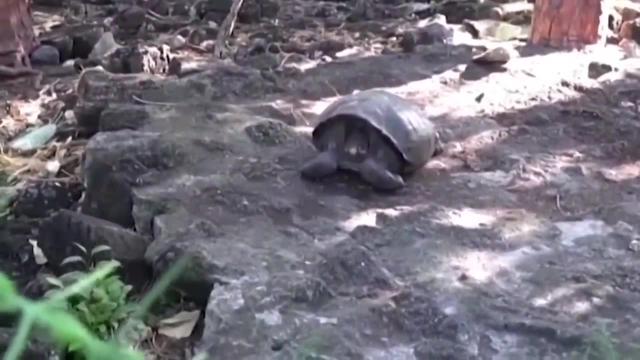 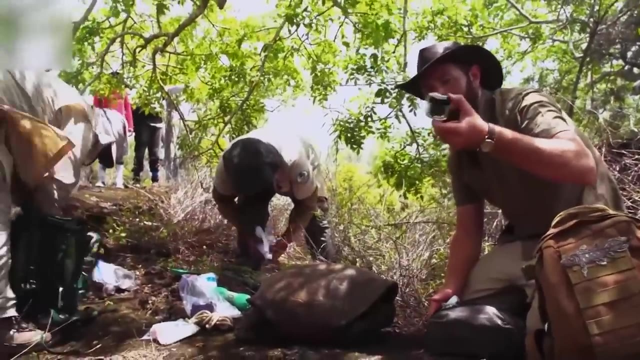 since 1906 until Fernanda showed up and blew everyone's minds Very slowly. Fernanda now lives at the giant tortoise breeding center on Santa Cruz Island, which is part of the Galapagos National Park. Recent expeditions found the tracks of two or three other tortoises that 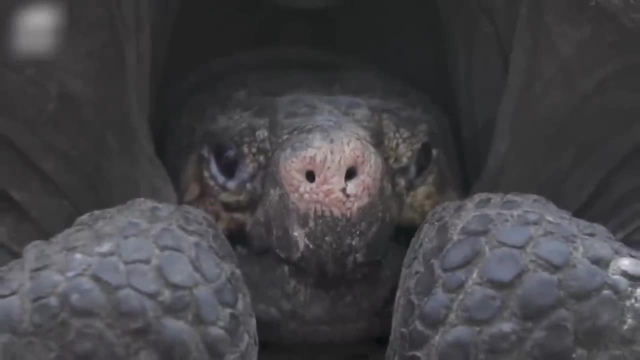 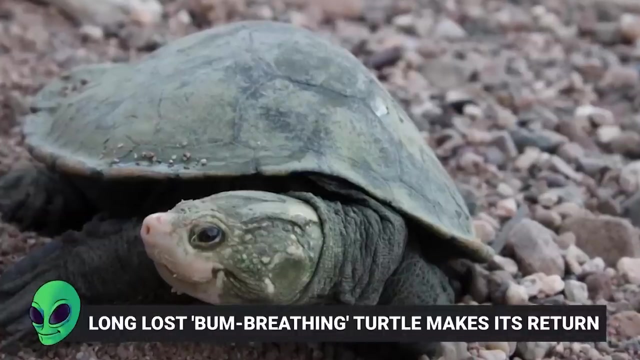 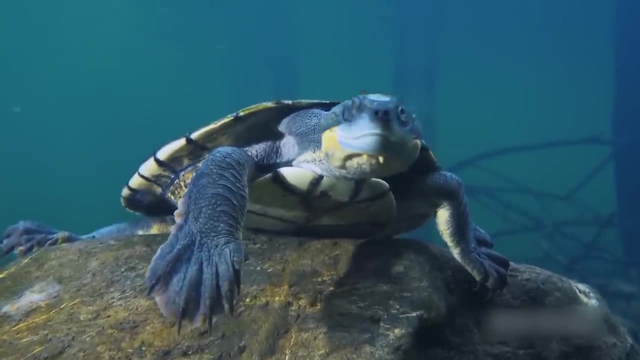 might be the same species. If this is true, it could lead local groups to think about starting a captive breeding and release program, Number 17.. Long-lost bum-breathing turtle makes its return. It's been 25 long years since this hard-to-find species was officially seen. 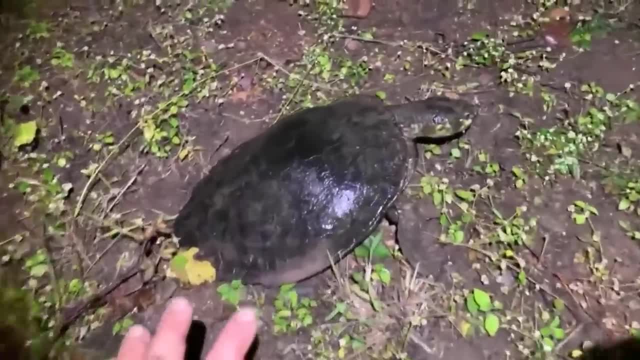 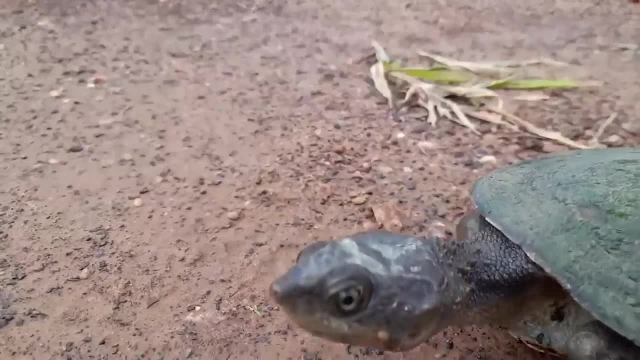 living in a small area along the Burdecan River on northern Queensland, But now a group of scientists and scientists have been able to find the tortoise. They've been able to confirm that Erwin's turtle lives not just at one site along the river but many sites along the. 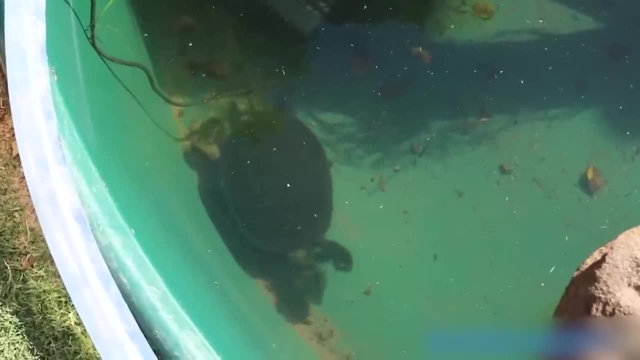 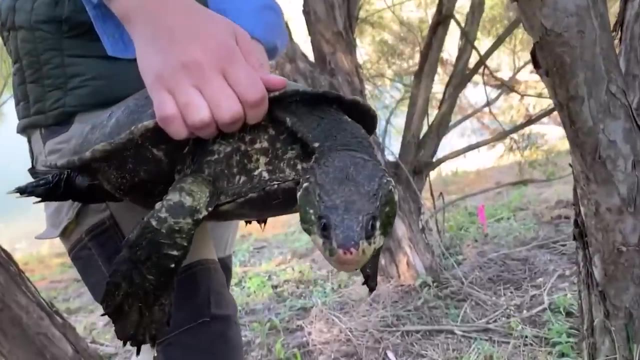 river. Stephen Bob Erwin found the turtle for the first time when they were camping on the banks of the Burdecan River and saw the turtle's pale colored face sticking up out of the water. This trait, which is caused by the lack of pigmentation cells near the skin surface, is what makes these 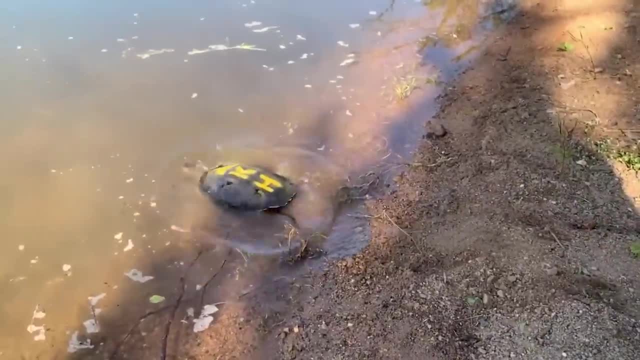 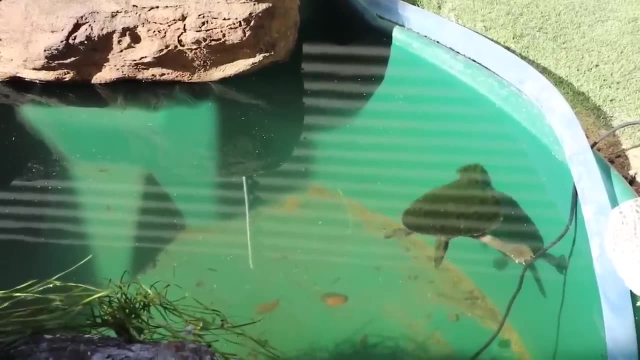 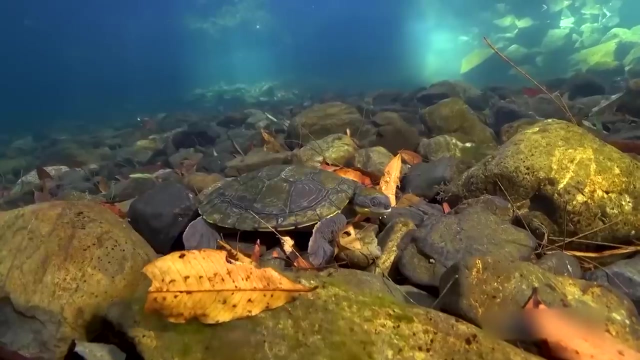 turtles special. That and the fact that they breathe through their butts. They're able to breathe underwater because they have a cloaca in the back of their bodies. This hole is also the digestive tract, the reproductive system and the urinary system. So yeah, these guys breathe through. 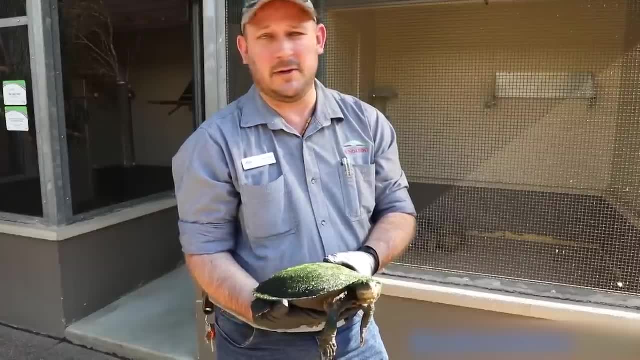 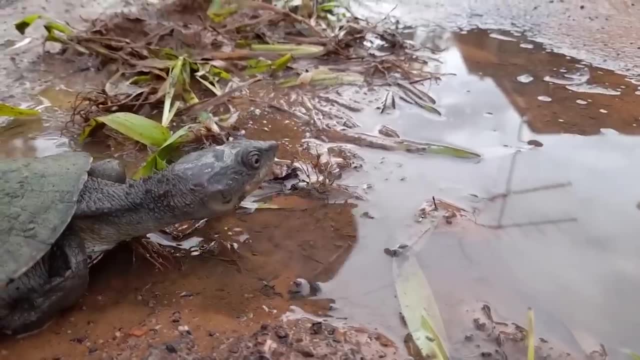 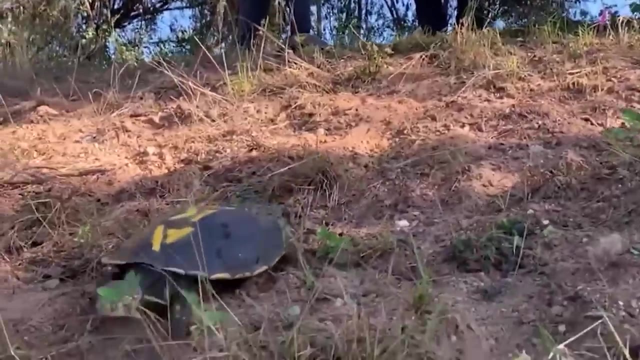 their buttholes. Erwin's turtle was found again thanks to new e-DNA detection technology used by a team of researchers led by James Cook University. They took the water samples from the lower Burdecan River and looked for environmental DNA in them. The river has changed a lot since the Burdecan Falls. 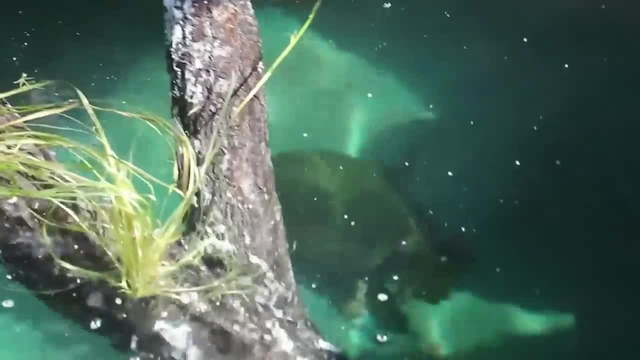 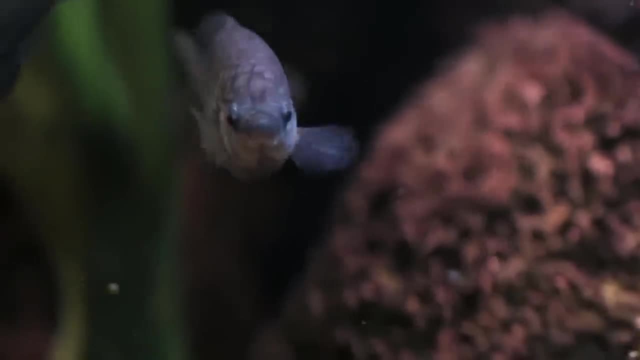 Dam was built, so it's a great place to live. Number 20. Long-lost bum-breathing turtle, So it's good to know that they're still there breathing through their buttholes. Number 16. Tequila fish: Marine experts thought that the tequila fish had gone extinct in 2003,, which was a shame, as it was. 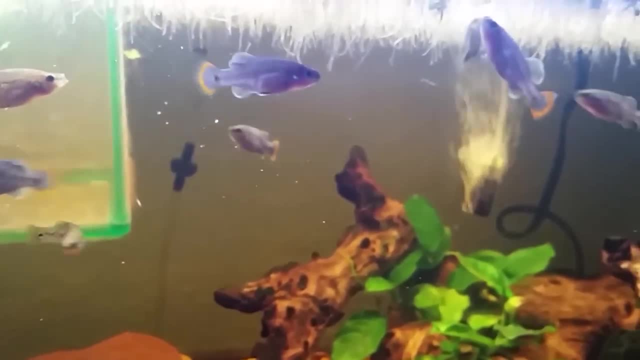 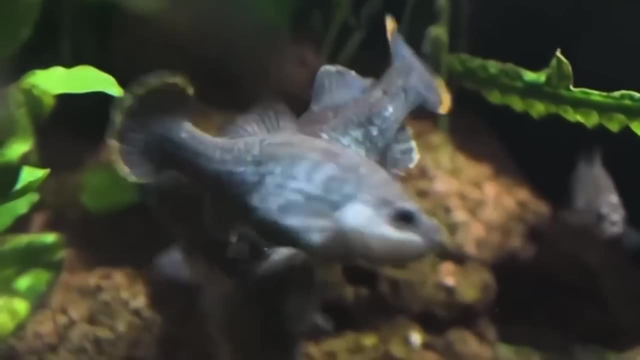 only discovered just a little bit before that Pollution and the spread of other exotic species into these waters were blamed for this, But experts at the Michoacana University of Mexico and Chester Zoo England worked hard to save the small fish species, and now they've been put back. 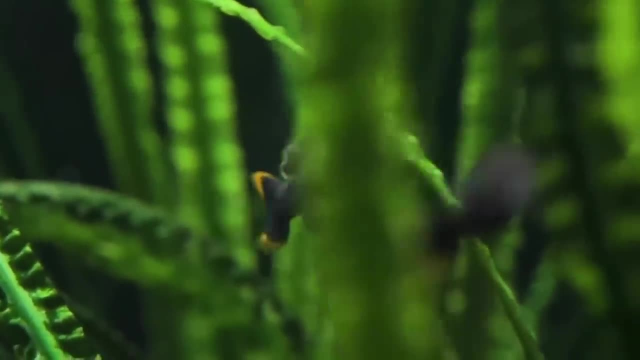 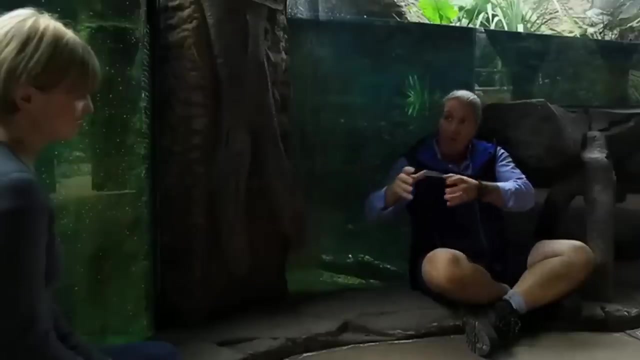 wild. In 1998, Chester Zoo gave 10 fish to the Michoacana University of Mexico. They were eventually set free in a man-made pond where the university staffed watch over them as they bred and formed colonies. After a few years, this number grew to thousands and it was decided. 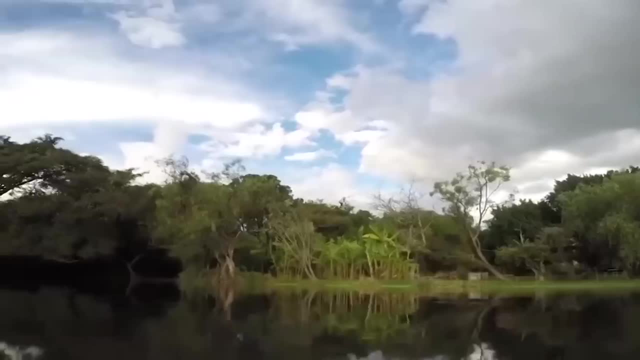 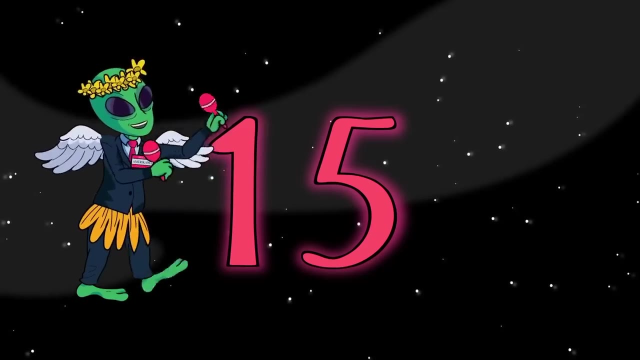 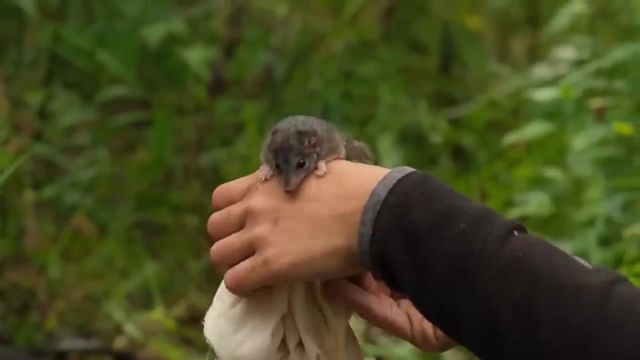 that 1,500 of these fish would be sent back to the Tuchitlan River in southwest Mexico, where the tequila fish population is now thriving. Number 15.. Silver-headed antichinus, Do you have way way too much testosterone? Are your balls hugely oversized for your body? Does 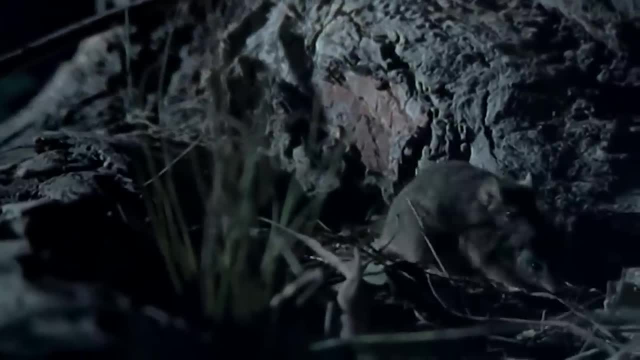 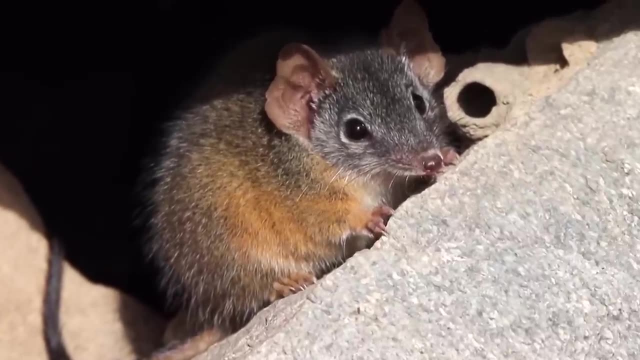 your body pump you full of the stress hormone cortisol. when you have s**t, which can cause internal bleeding, hair loss and even blindness, Do you still keep looking for females to mate with, even though you know it will kill you in the end? Well, if you said yes to all of the above, 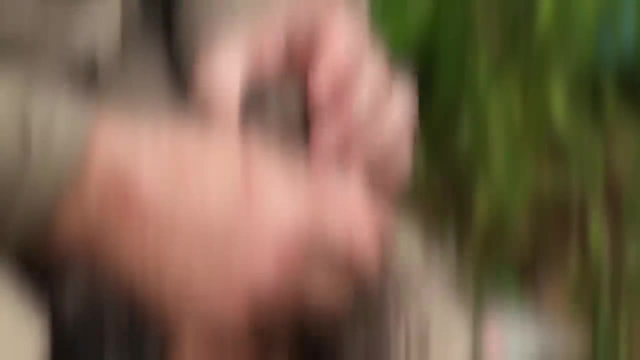 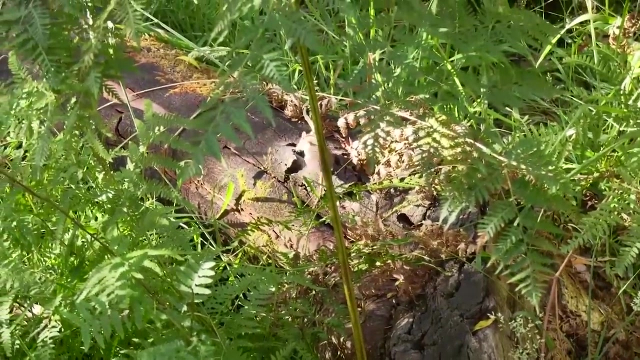 you're probably a male silver-headed antichinus, also known as a suicidal reproducer. If you said yes to all those questions and you're not a silver-headed antichinus, you're probably a male silver-headed antichinus. Get help now. There's a lot to learn about this small marsupial. 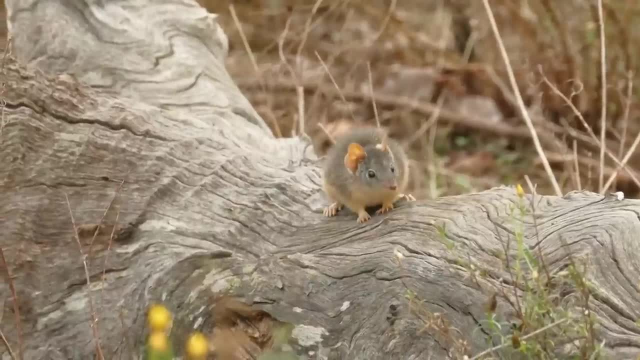 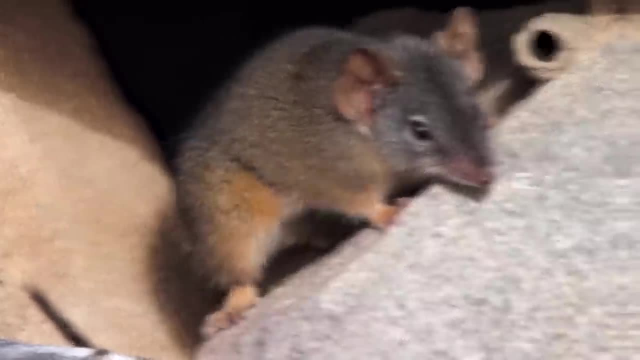 that looks kind of like a shrew. First, it's on the verge of extinction because of the 2019-2020 megafires. The silver-headed antichinus is one of the smallest marsupials in the world. It's only. 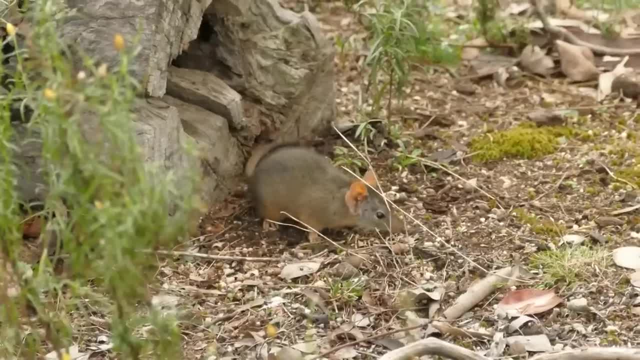 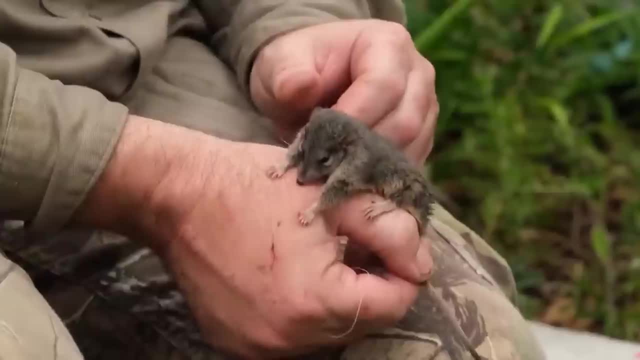 9 to 12 centimeters long. Even though they're small, they have big teeth that they use to eat spiders, cockroaches, beetles and other bugs that they find in the thick vegetation where they live. Before 2013, we didn't know that this kind of 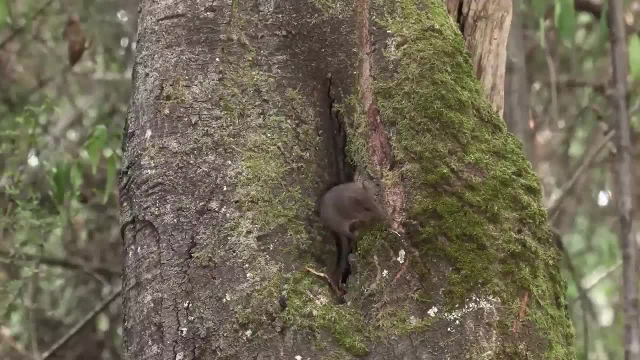 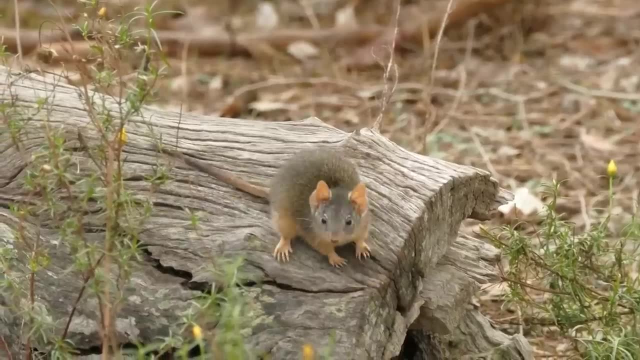 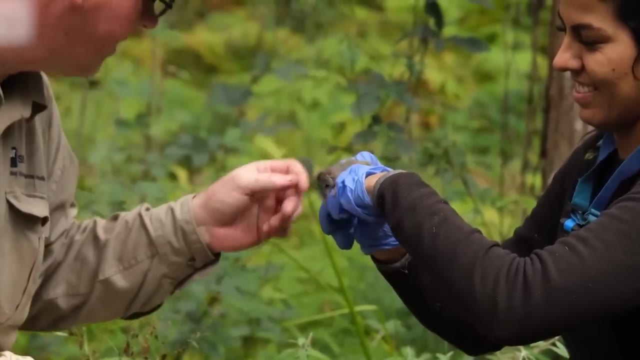 antichinus existed During mating season. the male's body gets so full of cortisol that it can go blind, lose all of its fur and start to bleed from the inside. Even so, it'll keep mating until it dies. It's a real romantic hero, Ladies, watch out. Either it cares more about the survival of 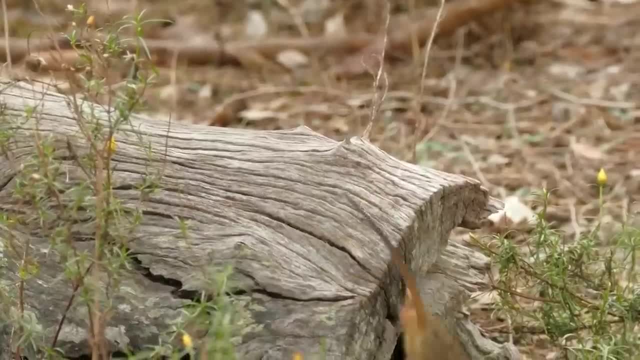 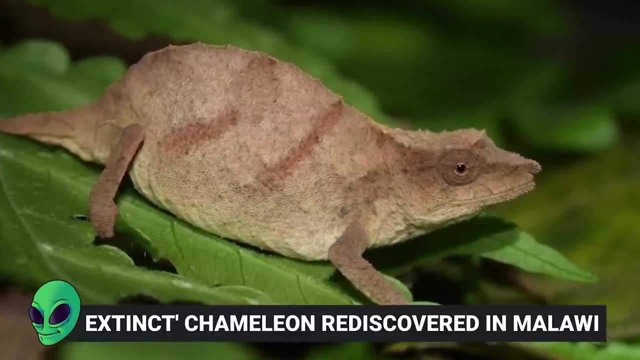 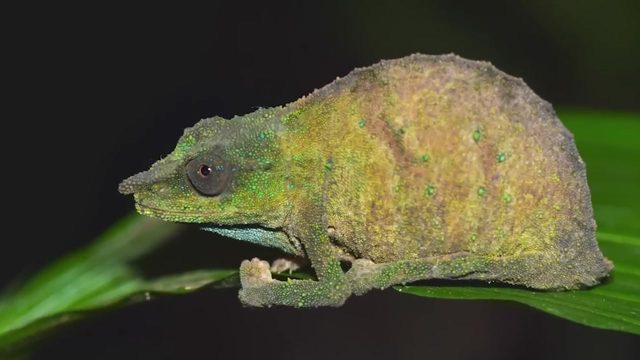 its species than its own life, or it's just really supremely horny and it wants to make love that badly. 14. Extinct Chameleon Rediscovered in Malawi. Next up the world's rarest chameleon. We thought it was extinct but it's been found again in a 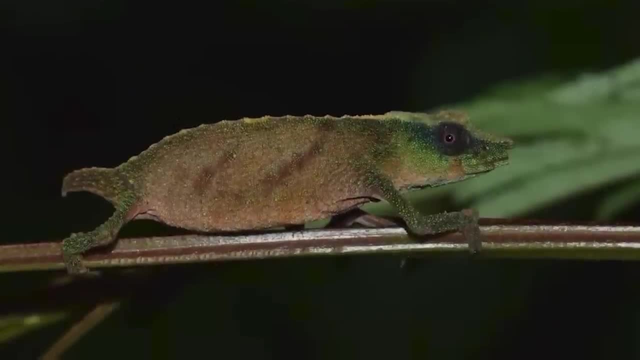 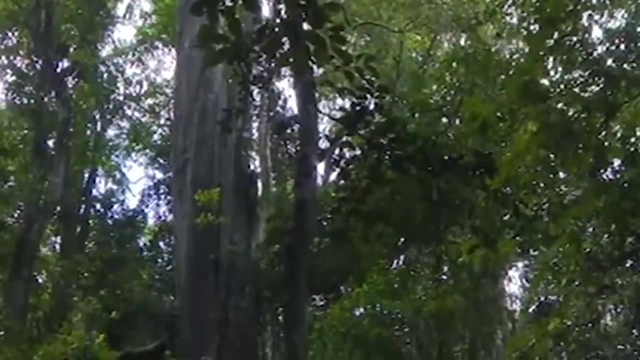 patch of forest in Malawi. The Chapman's pygmy chameleon is only 5.5 centimeters long and it's very rare. It lives on the low-elevation rainforest of the Malawi hills. It's losing its habitat. 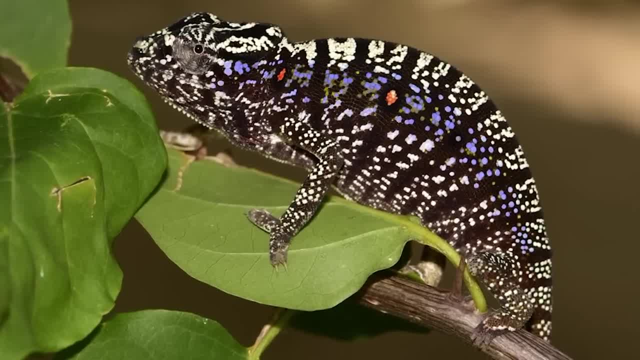 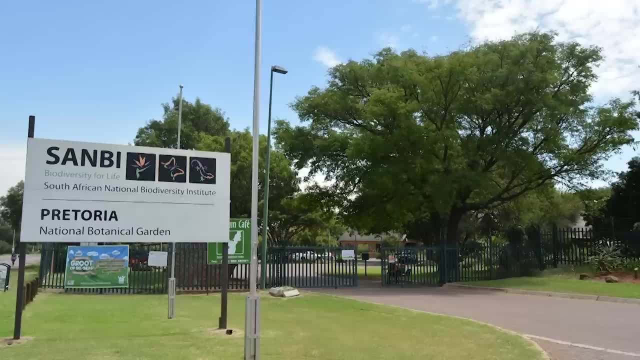 because people are farming more land in the region. Herpetologist Colin Tilbury wrote about the rare chameleon for the first time in 1992.. At the time, people thought that it had died out. However, researchers from the University of Malawi and the University of Malawi have found that the 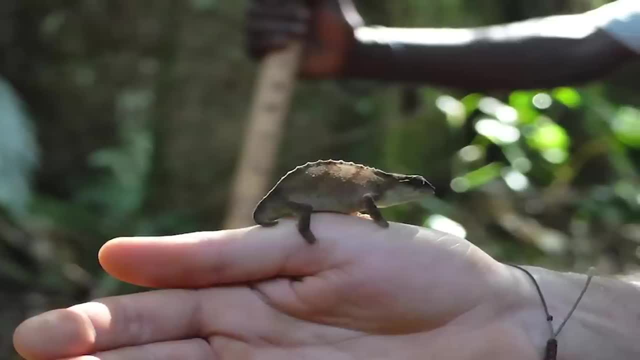 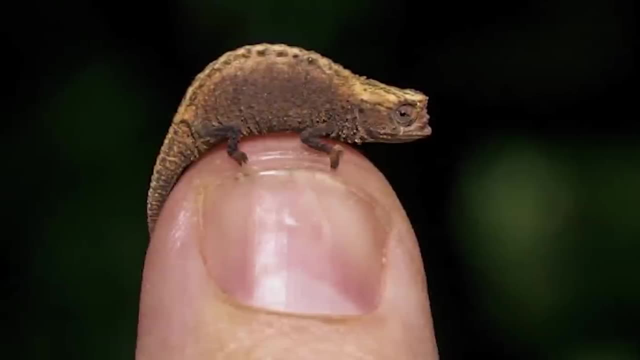 South African Biodiversity Institute did a survey in 2016,, and the results are just now being made public. for the first time, They found the small reptiles living in patches of the forest that hadn't been cut down. Other kinds of chameleons can be a little crazy, hissing and biting. 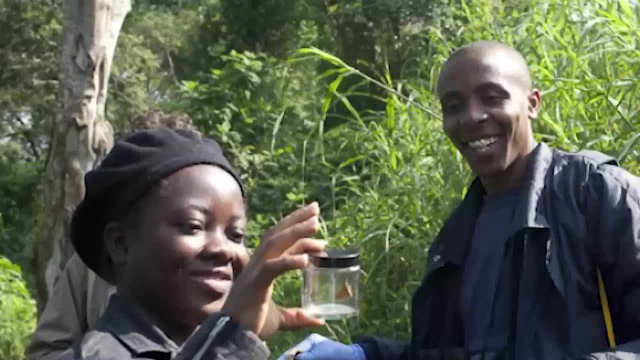 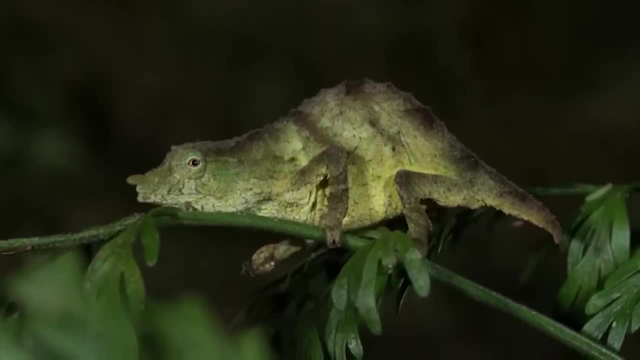 but pygmy chameleons are calm and real sweethearts. The team went back to the forest and found that the species was very rare but not extinct yet. They saw seven adult chameleons along a path in the first forest ten in a site six kilometers south of Malawi. The chameleons were found in a. 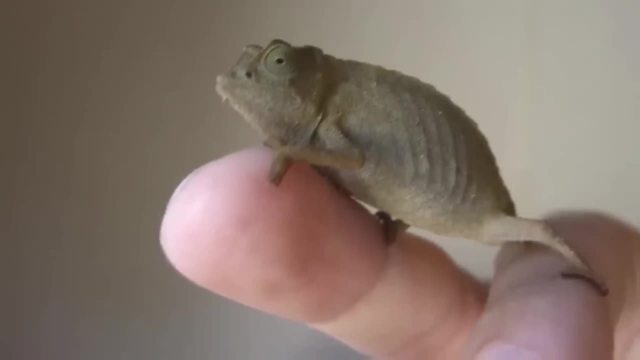 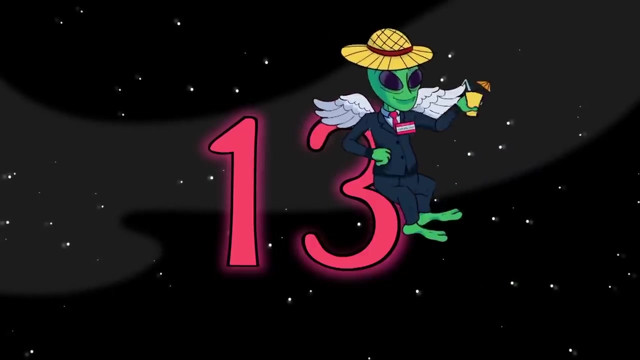 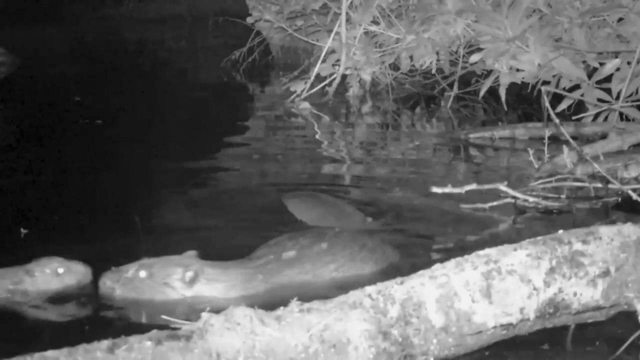 forest patch near Mekundi where 37 chameleons had been released in 1998 to try to protect the species Number 13.. First Baby Beaver Born in Exmoor in 400 Years. A baby beaver, also called a kit, has been born in Exmoor, UK, for the first time in 400 years. 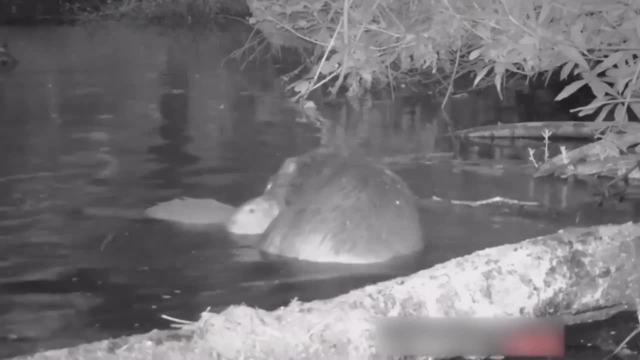 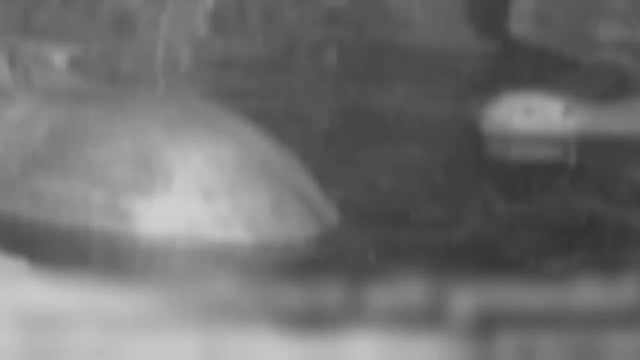 Since it was born, the beaver, which was named Rashford, has been seen with its parents many times on the National Trust's Honeycutt estate. The beaver was born in Exmoor UK, for the first time in 400 years. To celebrate, a conservation charity put out new footage from a stationary. 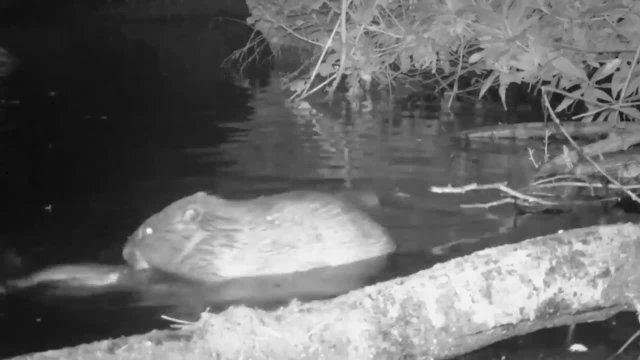 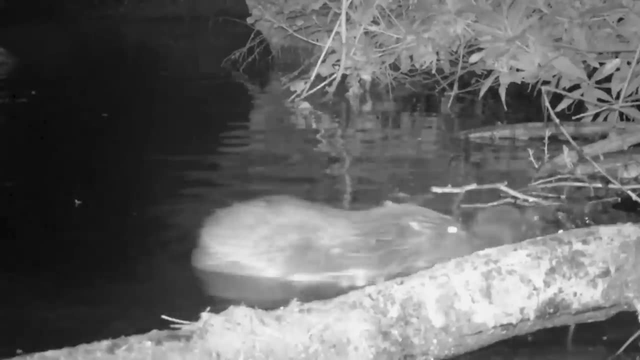 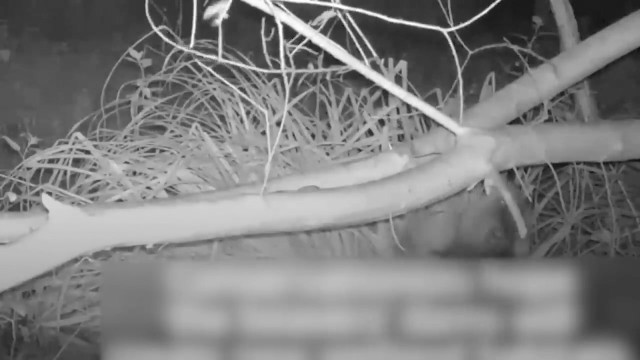 camera that shows Rashford, who's one years old, building a dam and moving mud with his dad, Yogi. Grylls and Yogi, the parents of the kit, got together in 2020 after a conservation charity got its first license to let the Eurasian beavers live in a specially built 2.7 hectare enclosure. 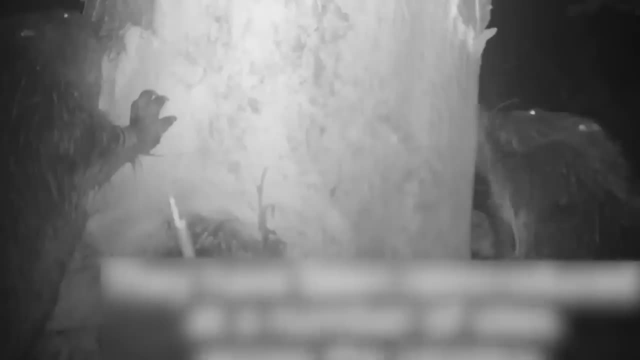 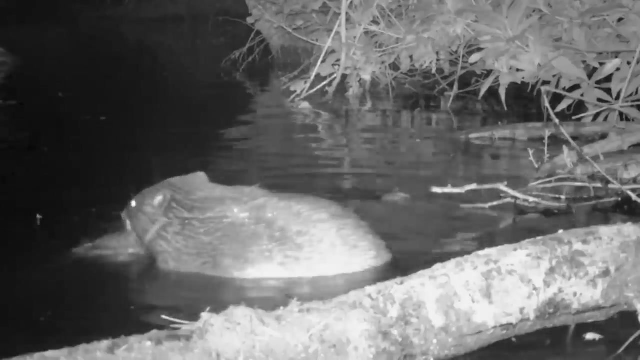 in Honeycutt. After the birth was announced, thousands of people on social media voted to kit Rashford. They were inspired by how well the England team did at the UEFA European Football Championships that summer and so named the little guy after one of the star soccer players. 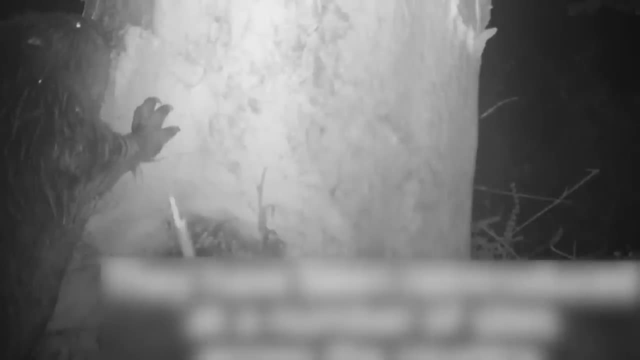 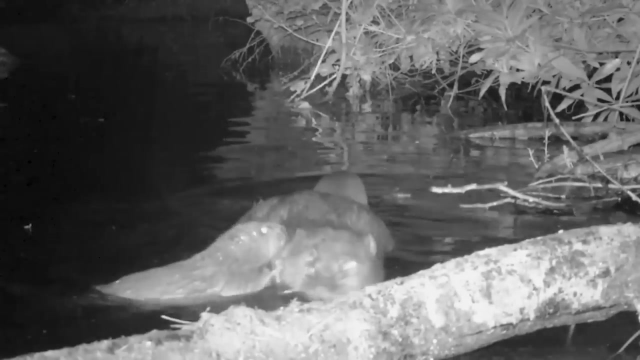 Since then, young kit has been helping its parents turn the unmanaged woods into a more open wetland where more animals can live. We hope that Rashford will be one of the first of many kits to be born at Honeycutt, and early signs suggest that more kits may be on the way. 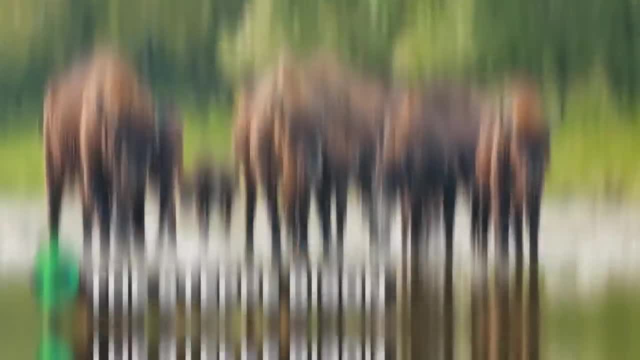 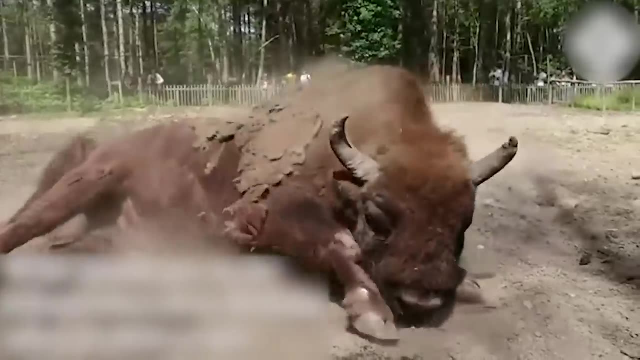 Number 12.. The Step Bison Rashford isn't the only animal making a comeback in the UK. For the first time in 6,000 years, wild bison will be back in Great Britain In the spring of 2022,. a small herd was set free in Kent. 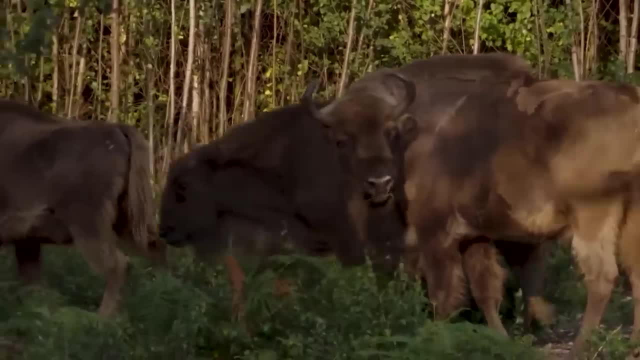 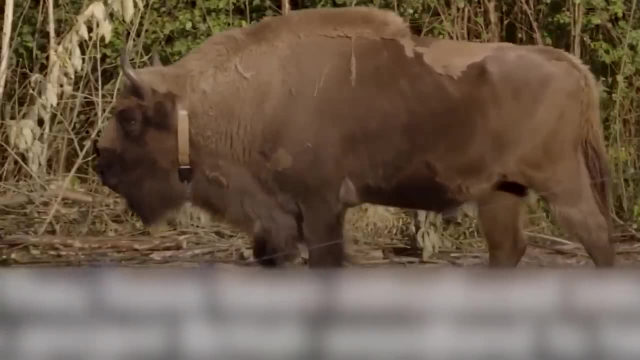 One male and three females were set free during the first release. Lucky guy with three ladies to choose from. The herd will then grow through natural breeding, and each female usually has one calf per year. The bison will come from the Netherlands or Poland, where they've been. 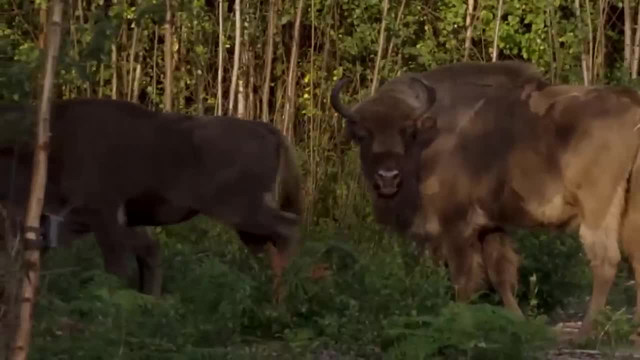 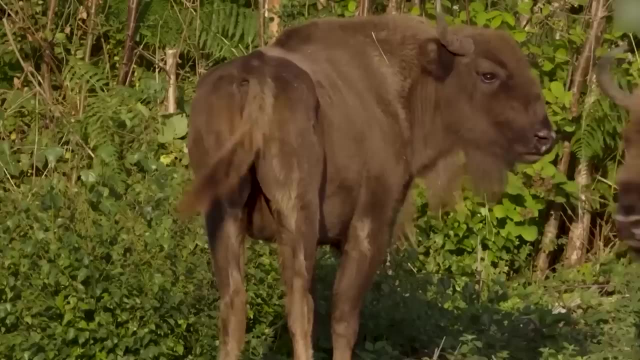 released safely and with good results. Since then, they've been in the wild for a long time, and the number of UK's most important animals has dropped by an average of 60%. Even though conservationists work hard, England is one of the countries with the least amount of 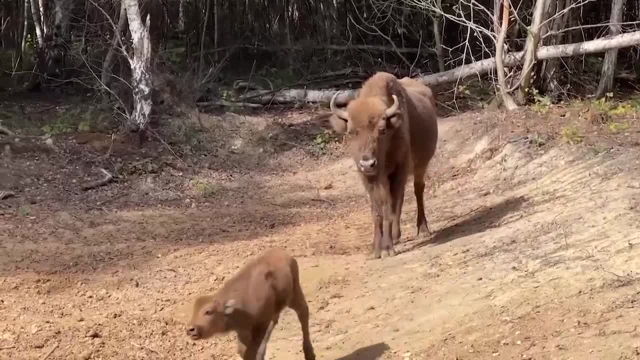 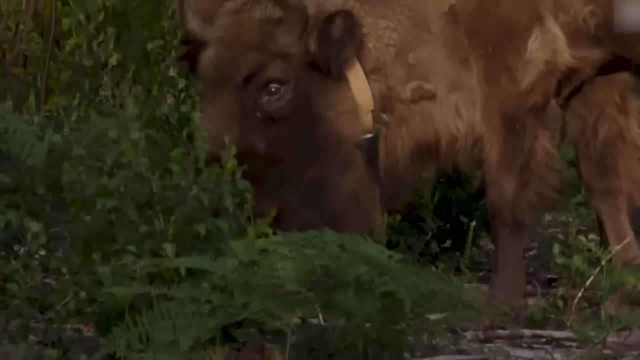 nature left. Bison kill certain trees by eating their bark or rubbing against them to get rid of their thick winter fur. This makes dead wood a feast for insects, which in turn feed birds. When trees are cut down by bison in this natural way, they make way for sunny areas where native 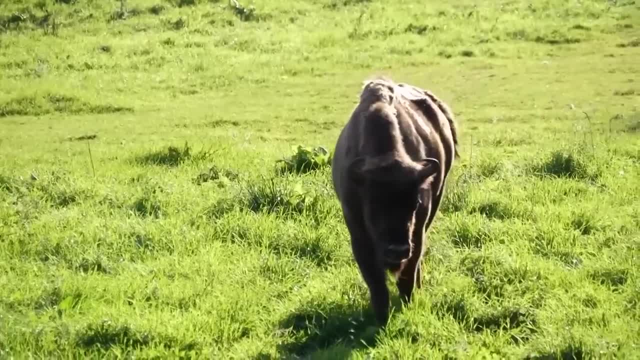 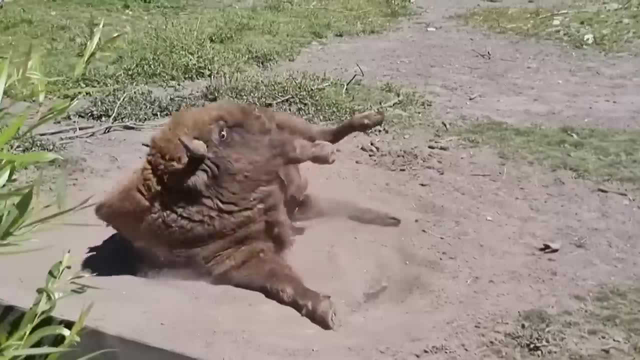 plants can grow. The Trust thinks that the bison's eco-standardism is a good thing. It's a good thing because it will help birds like the nightingales and turtle doves. People think that the steppe bison lived in the UK until about 6,000 years ago, when hunting and changes in its habitat killed it. 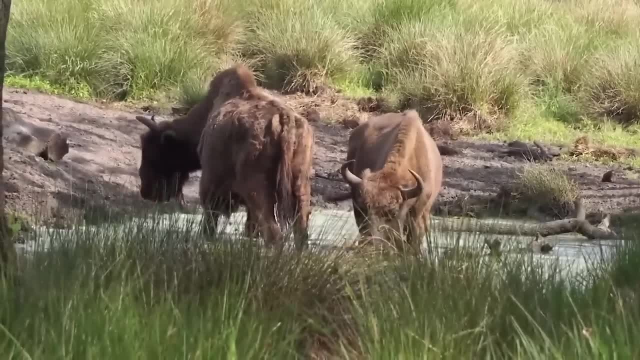 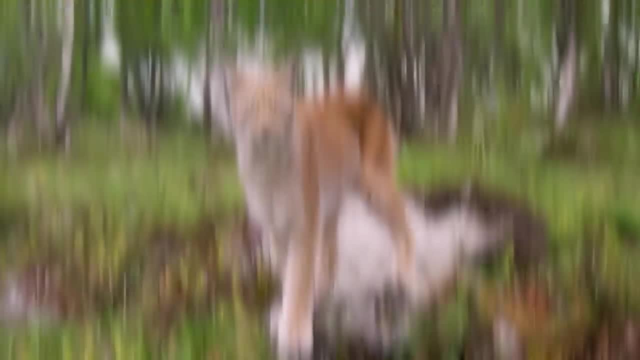 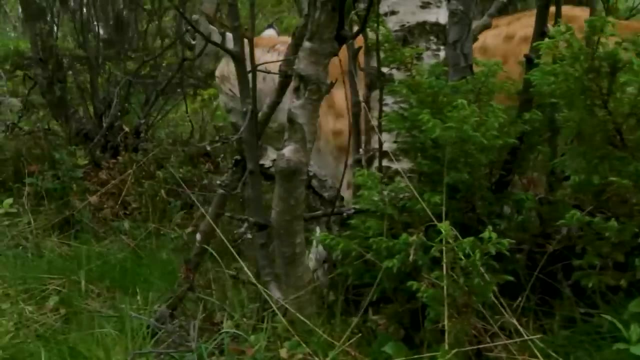 off This species' closest living relative, the European bison, is a descendant of this species. 11. Eurasian Lynx. The normal range of the Eurasian lynx is pretty big. It goes from Western Europe to Central Asia. Its original range, on the other hand, is about 1,000 feet long, So it's a pretty big bison. 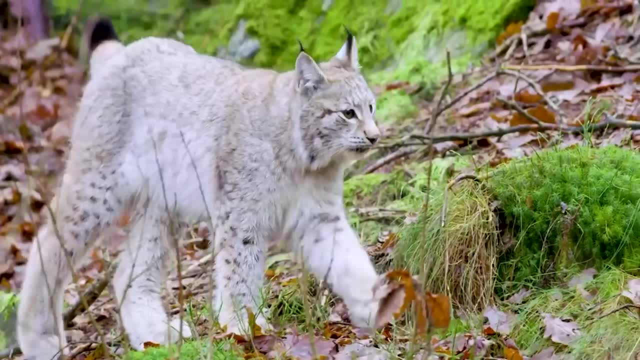 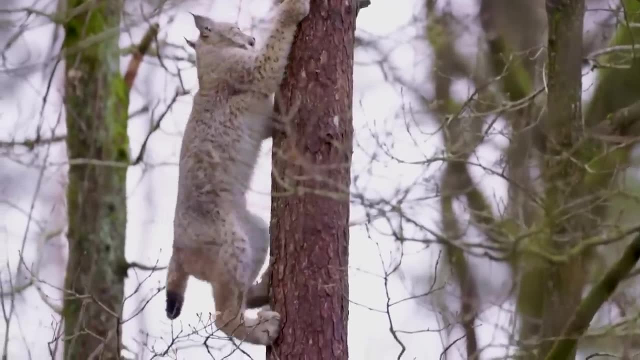 It has shrunk a lot in the last few hundred years, And in Central Europe only small groups of them have survived because of people trying to kill them. There are still a lot of lynx living in the Baltic Scandinavia and the Carpathian Mountains. 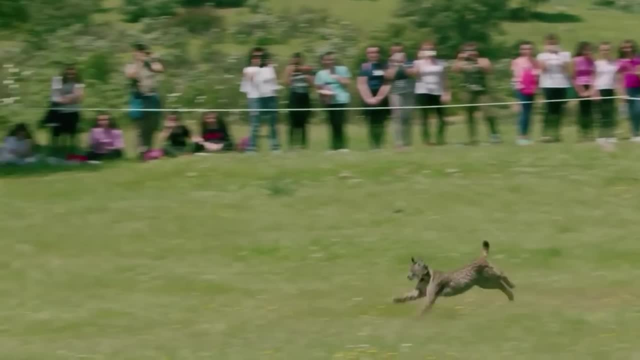 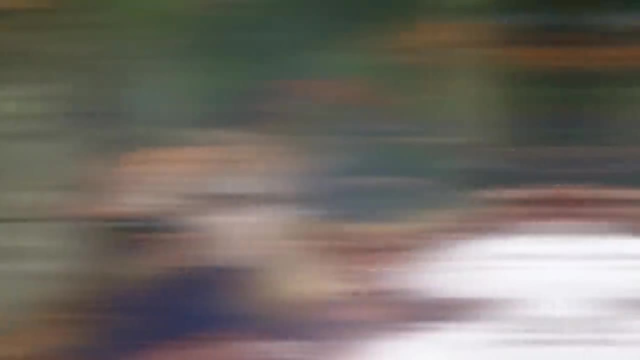 The Balkan lynx is a rare subspecies of the Eurasian lynx. It's thought that less of 50 of them are still alive. So the Balkan lynx is one of the most rare cats in the world. It only lives in the southwest part of the. 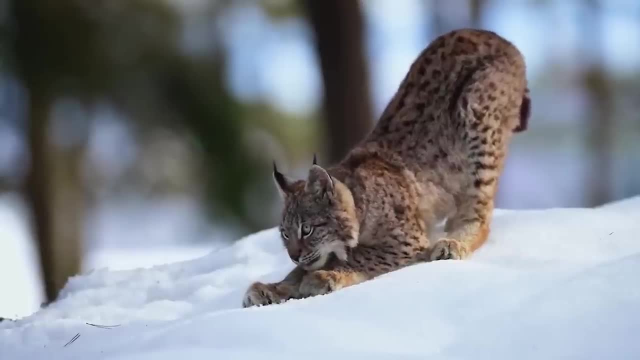 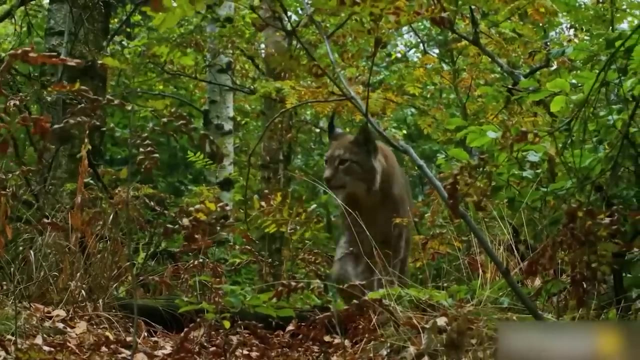 Balkans, But the Balkan lynx is having a hard time there because its habitat is being destroyed and it's being directly hunted even today. Since the 1800s, the Eurasian lynx hasn't been seen in Central Europe, but it's finally returned to Switzerland, France, Italy. 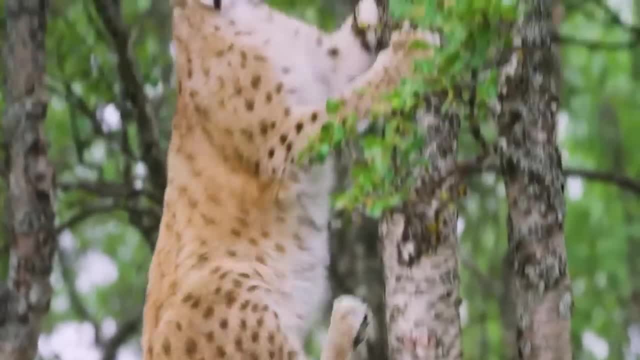 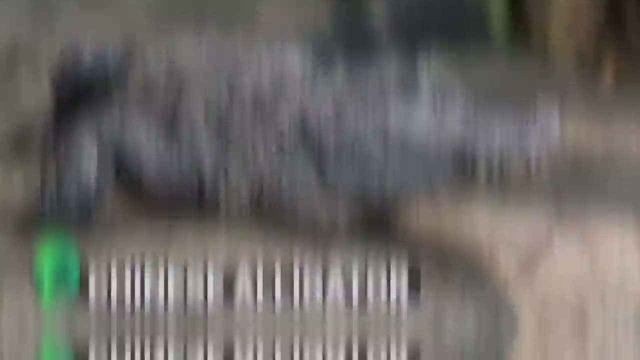 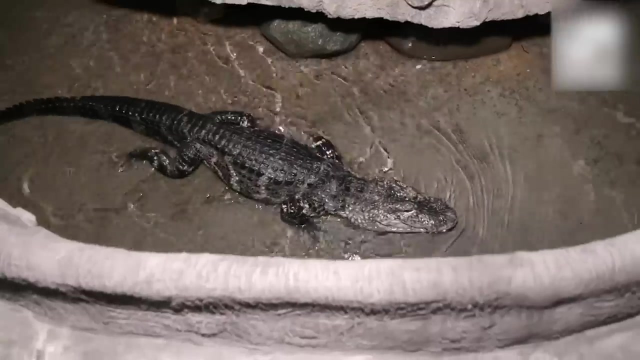 Austria and Germany, among other places. So maybe this is the start of a new era for this mysterious cat. 10. Chinese Alligator. The Chinese alligator, which is nearly extinct, is different in several small ways from its American cousin: It's smaller, has a bigger head. 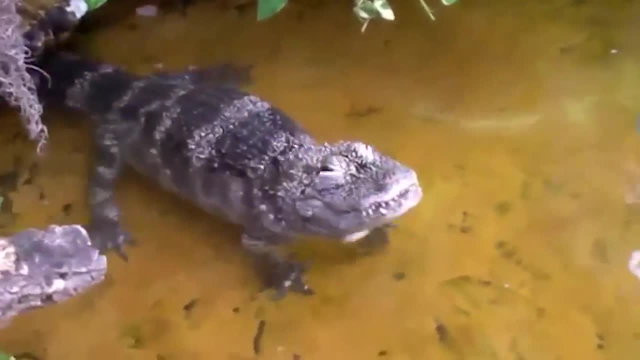 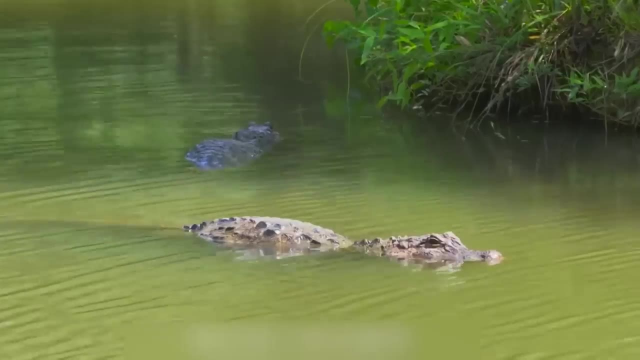 and its nose is a little bit turned up. The American alligator doesn't have a plate of bone on the inside of its eyelids like the Chinese alligator does. The Chinese alligator also has bony plates on its belly, called osteoderms, which the American alligator doesn't. 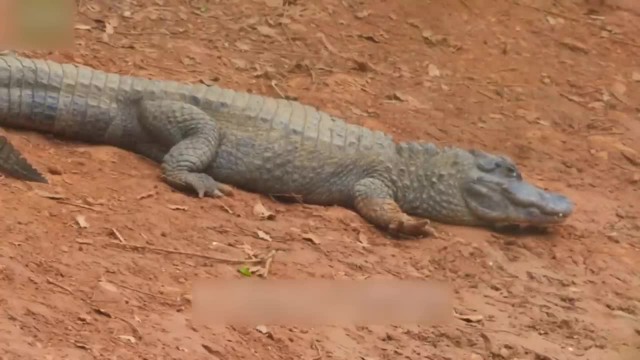 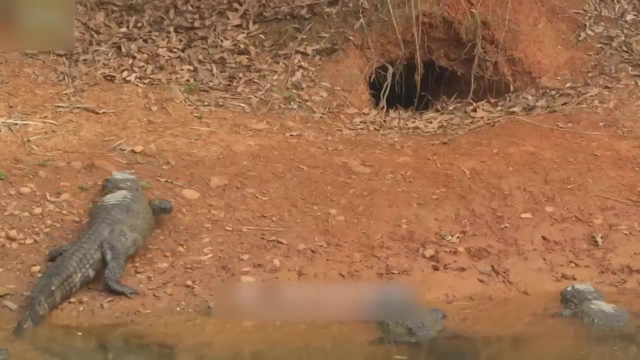 have. The Chinese alligator is the only member of the family Alligatoridae that doesn't live outside of the Americas. in fact, In the past, the Chinese alligator lived in the many, many lakes and marshes along the middle and lower Yangtze River, from Shanghai to Jianling City in 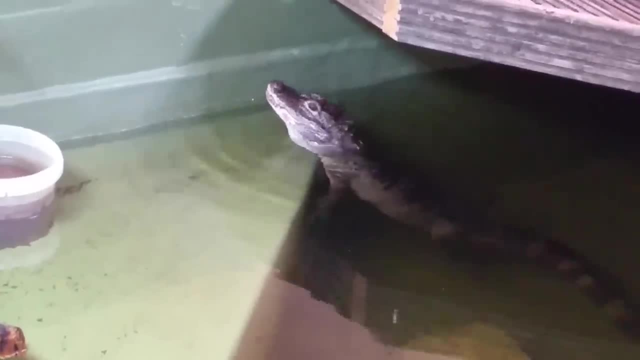 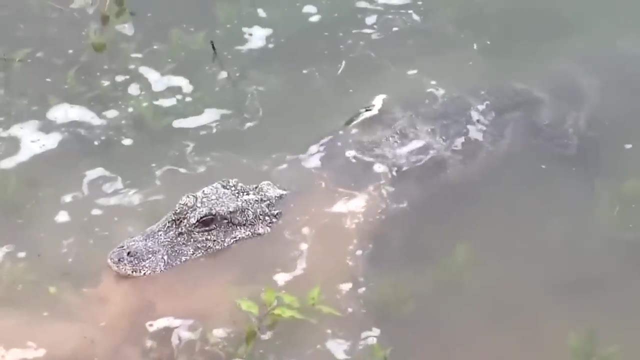 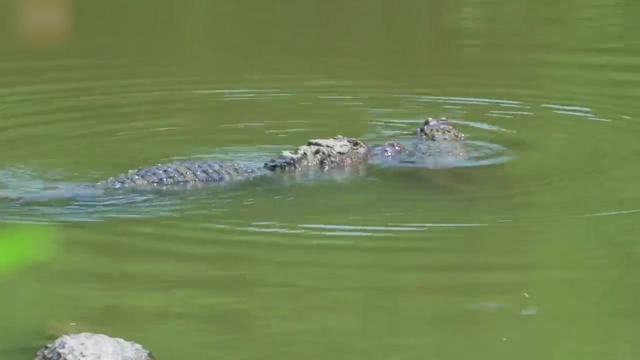 the Hubei Province. It's now only found in the lower Yangtze, mostly in the providences of Anhui and Xinjiang in eastern China. The Chinese alligator used to be found all over the Yangtze River basin, but now there's few of them. In 1999, a survey found about 100 animals in the wild. 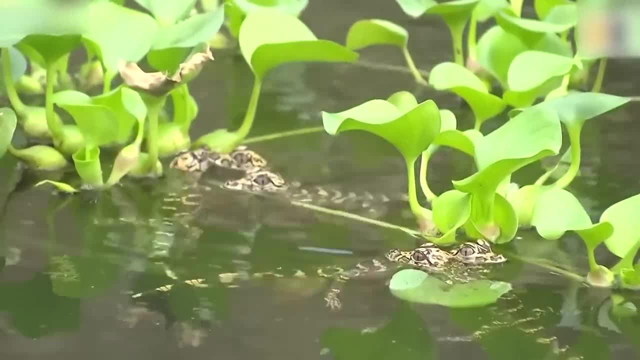 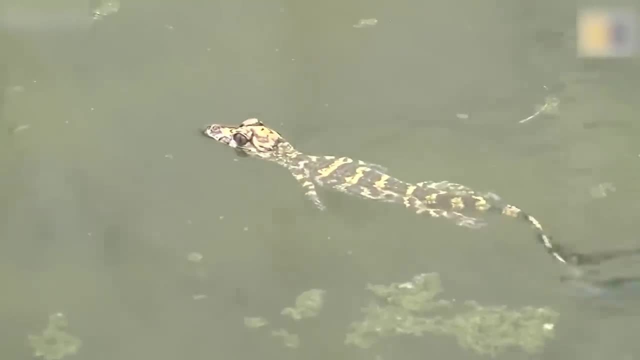 and only 10 places, But in 2001, programs to breed animals in captivity and put small numbers back into protected areas began. In 2019, another 120 alligators were set free, which more than doubled the amount of wild alligators. so things are starting. 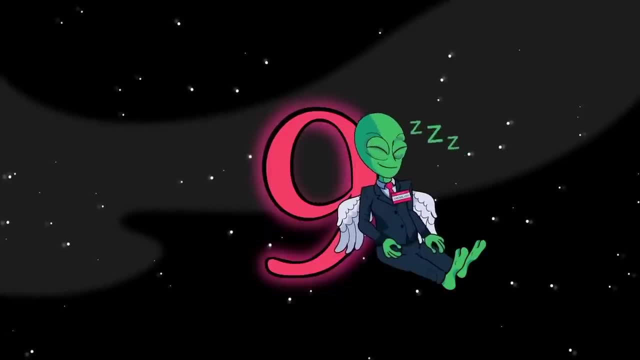 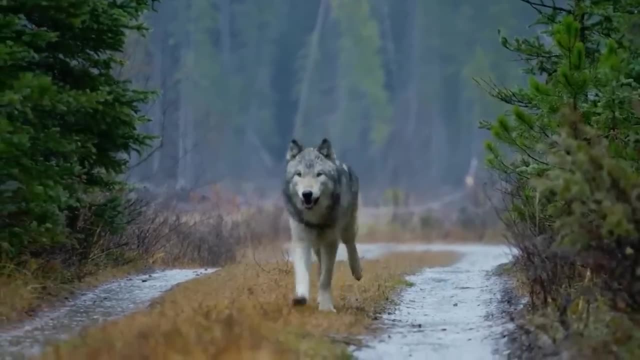 to look up for this rare gator at last. Number 9. Grey Wolves. When the grey wolf was brought back into the Greater Yellowstone Ecosystem in 1995, there was only one beaver colony in the park. Today there's nine beaver colonies in the park. 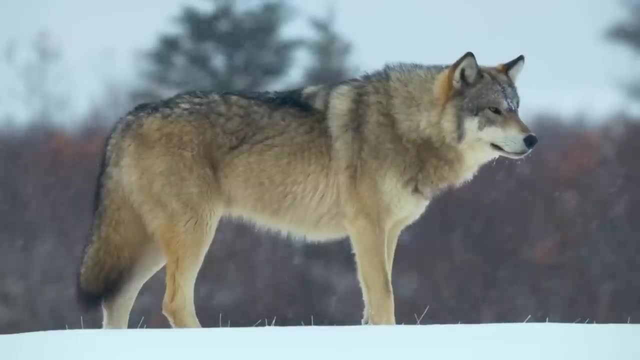 and there may be more in the future. The reintroduction of wolves continues to be a major challenge for the Chinese alligator, and the Chinese alligator is one of the largest beavers in the world. The Chinese alligator is a species that continues to surprise biologists with its direct and indirect effects on the 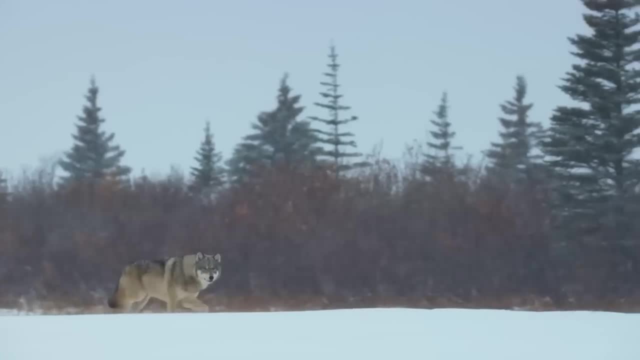 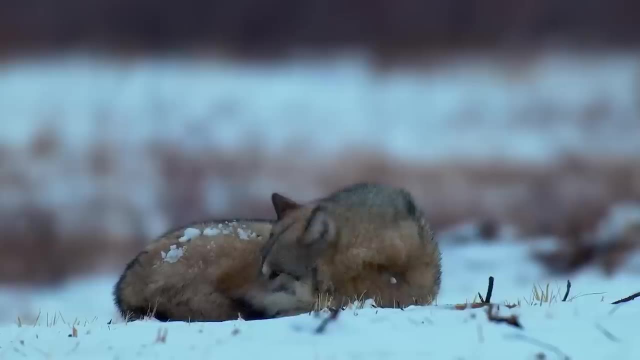 ecosystem as a whole. What happened was that the wolves set off a chain of changes in animals and plants that are still happening and will take decades of research to figure out. So how did this huge amount of change affect the beaver? To find out, we have to go all the way back to 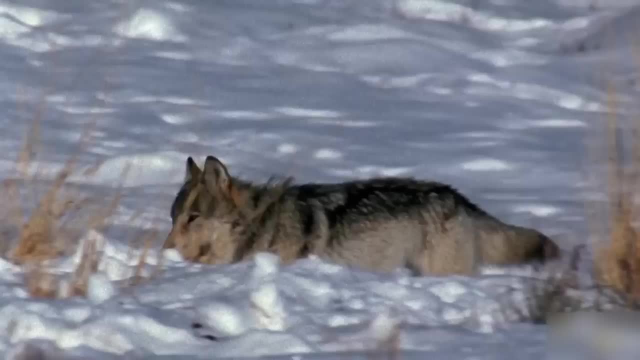 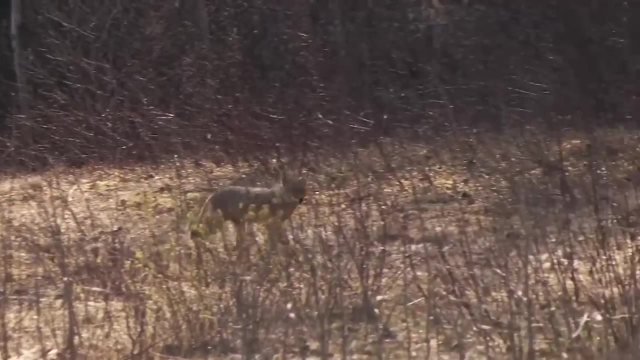 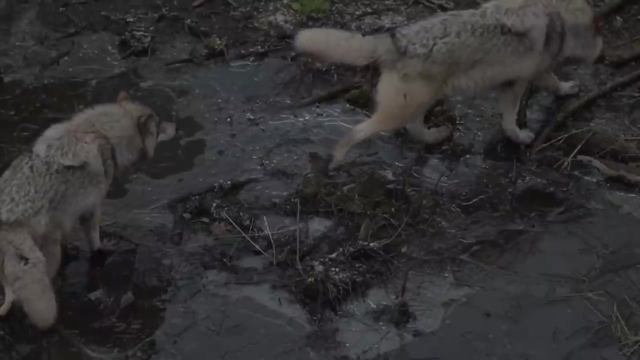 the 1930s, when all of Yellowstone's wolves were killed, Even though black and grizzly bears, cougars and, to a lesser extent, coyote still hunted Yellowstone elk, the lack of wolves took a huge amount of pressure off the elk. Because of this, there were a lot of elk, maybe too many. The elk pushed. 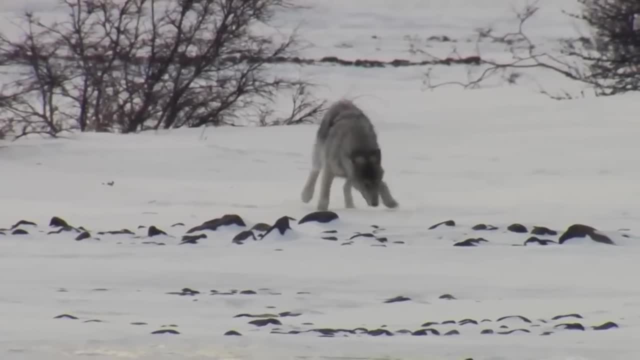 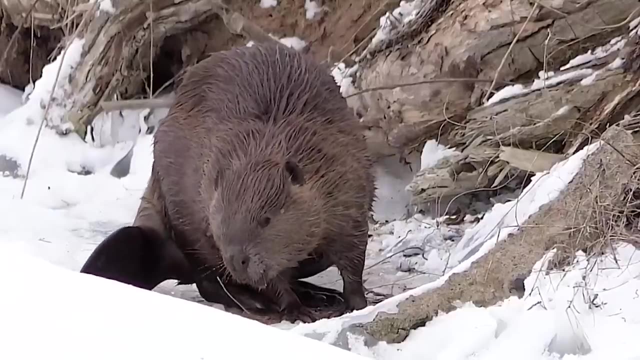 Yellowstone's carrying capacity to its limits, and they didn't move around much in the winter. Instead, they just spent most of their time eating young willow, aspen and cottonwood plants. Beavers had a hard time with that, because they need willows to live in the winter. 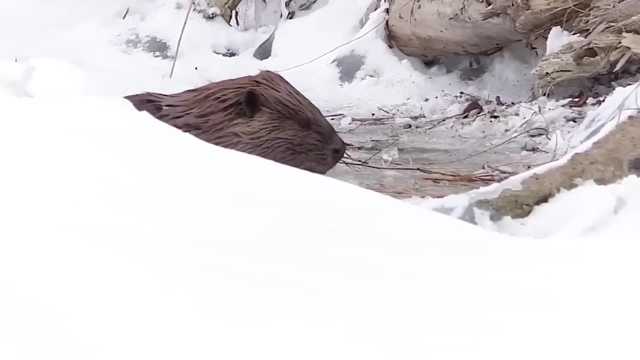 So was the answer to reduce the elk population? Well, no, in fact, In 1968, when the Chinese alligator was killed by a wild boar, it was said that it was the best way to kill a wild boar. 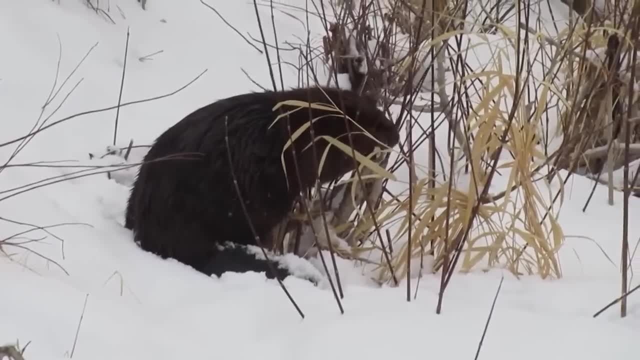 In 1968, when the Chinese alligator was killed by a wild boar. it was said that it was the best way to kill a wild boar In 1968, when there were about a third as many elk as there are now. 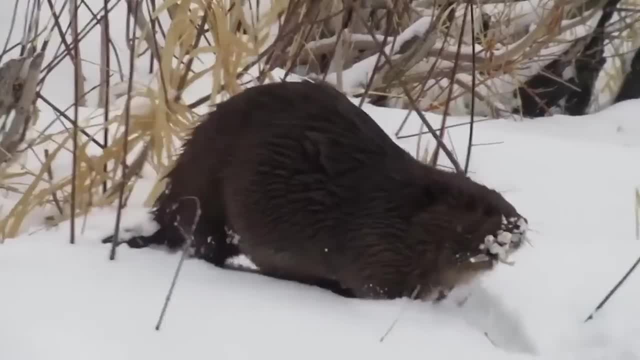 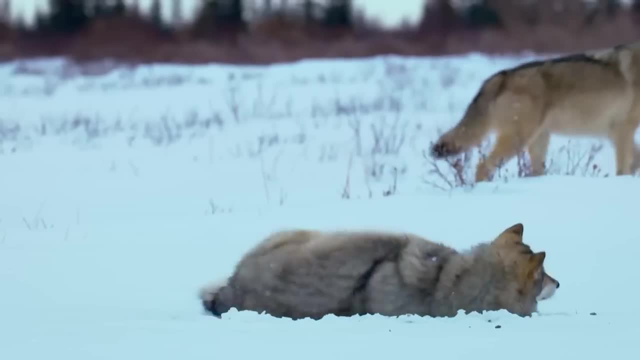 the willow stands on the streams were in bad shape. Now that there were three times as many elk as before, willow stands are strong, So how could this be? Well, it's because wolves are predators. They keep the elk moving. 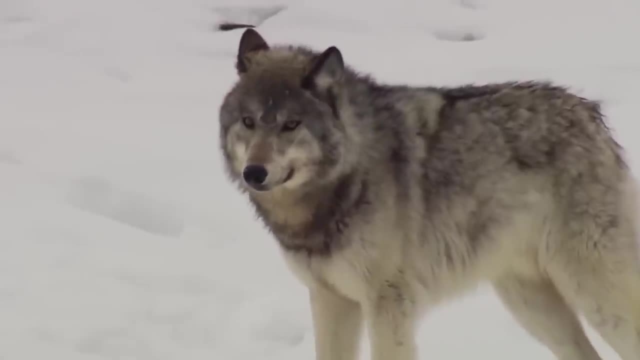 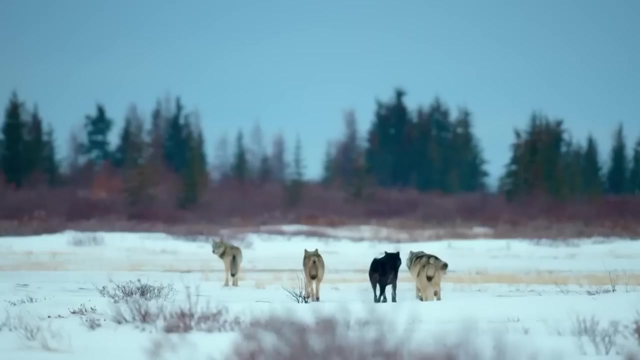 so they don't have time to graze the willow too much, no matter how many of them there are. As elk moved around more during the winter, due to nearby wolves, willow stands recovered from being heavily browsed and beavers found a lot of food that wasn't there before. We kind of touched on. 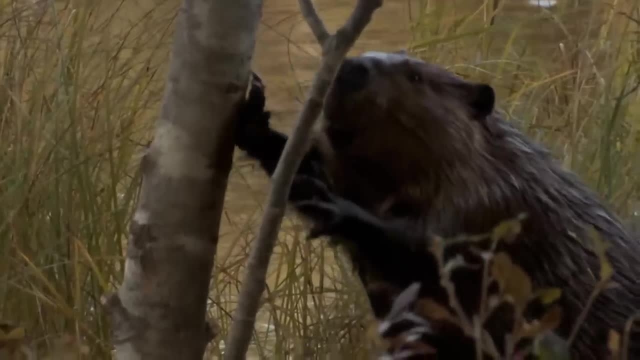 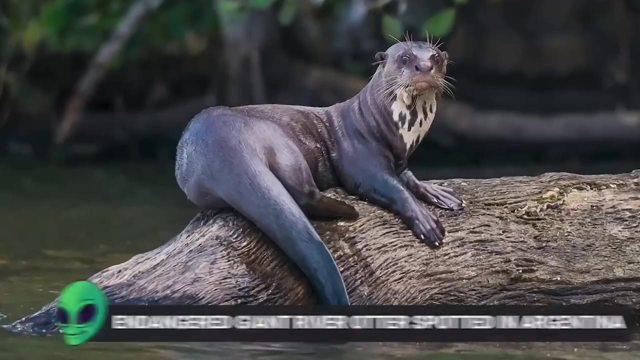 this earlier with another story. but beavers do a lot to the ecosystem and all of a sudden you got this huge chain reaction just from adding in some wolves. 8. ENDANGERED GIANT RIVER OTTER SPOTTED IN ARGENTINA. 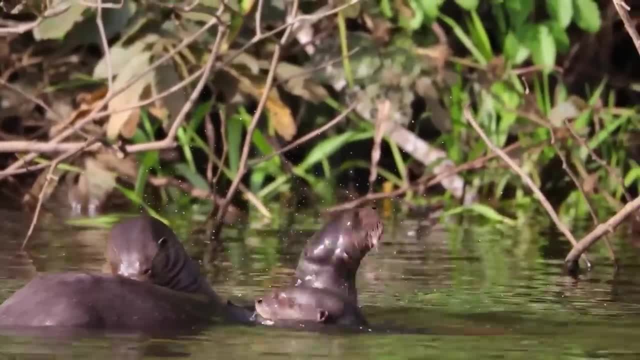 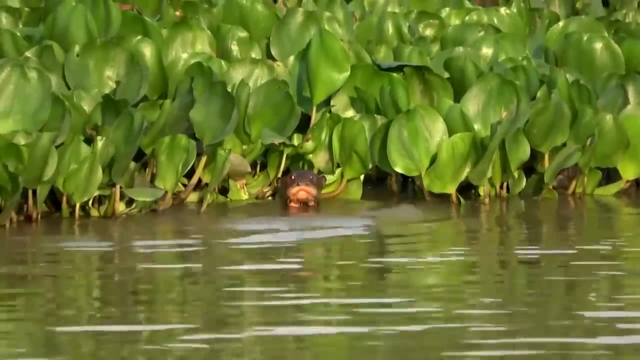 Before it was recently spotted again, people thought the giant otter had died out in Argentina because habitat loss and hunting made it hard for them to live. These otters are really huge and can be up to 1.7 meters long, making it the world's biggest otter. 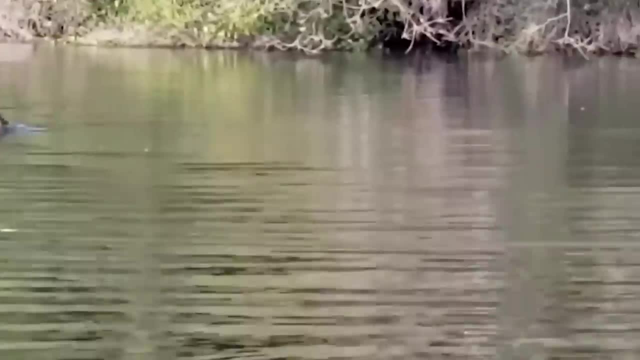 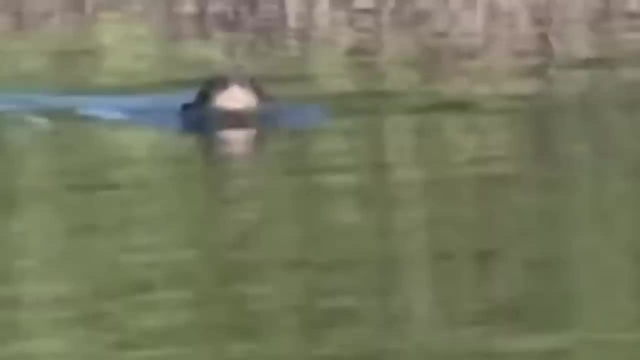 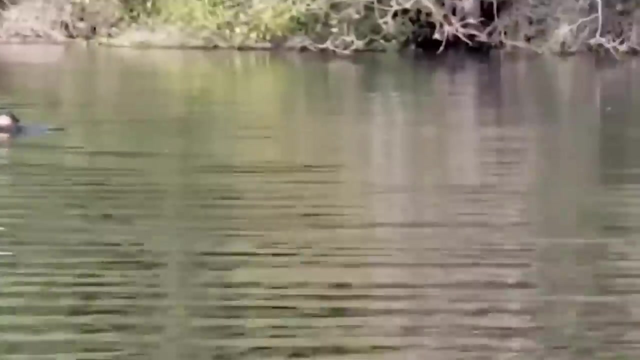 In May of 2021, while kayaking on the Bermejo River in El Impenetrable National Park in the Chaco Providence of Northeast Argentina, a nature specialist took a picture of a single male giant otter with his phone. The nature specialist had the phone, to be clear, not the otter. 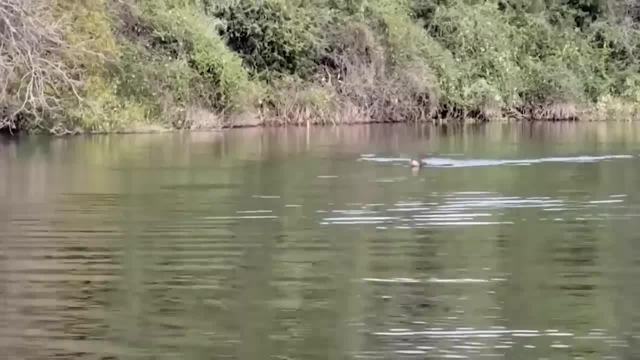 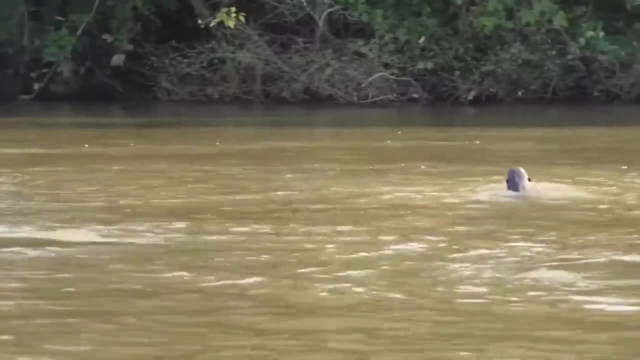 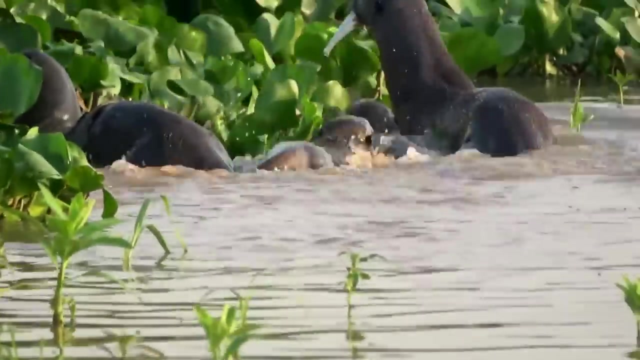 He wasn't looking for or expecting to see this animal, but he was very happy to see the amazing otter, which can be up to 30 kilograms, back in the Bermejo 9.. GIANT OTHERS. These giant otters are major predators in the waterways of South America. They're awake during. 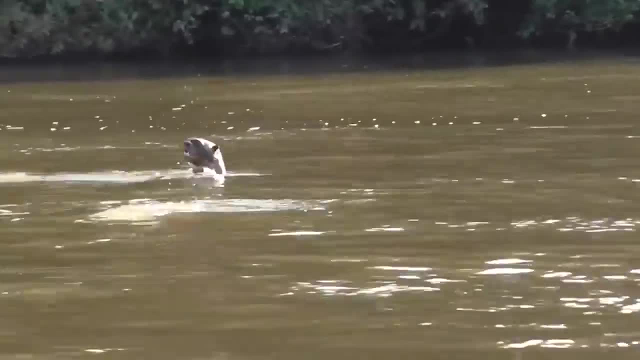 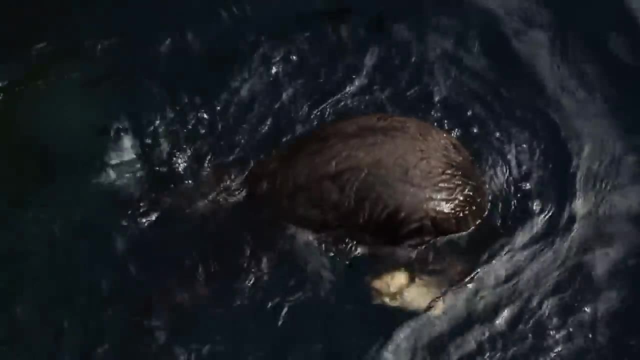 the day, make a lot of noise, are friendly to people and are very active. They never stop moving and love getting in and out of the water in funny and cute ways. That's another reason why they died out: because humans see something friendly and cute and funny and their first. 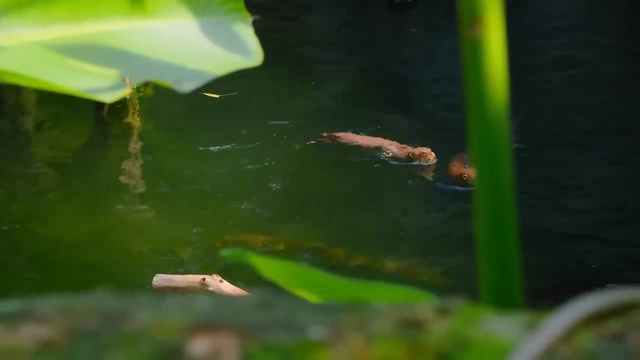 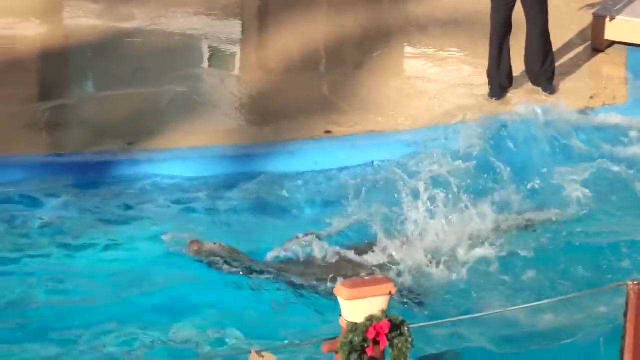 thought is to blow it up to pieces with a shotgun, which is exactly what happened. Loads of humans lining up to blast the giant otters, adults and babies alike, until they were finally near extinction. What a lovely species we are. 7. PIGMY TARSIER. 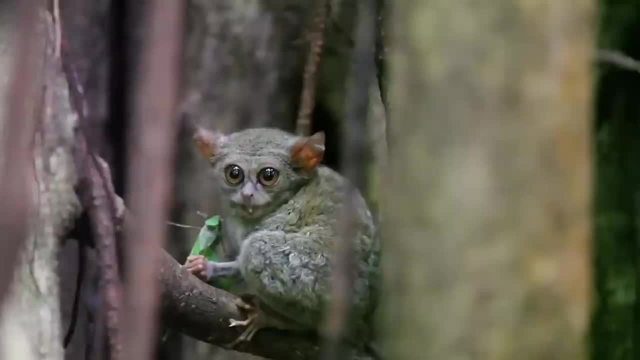 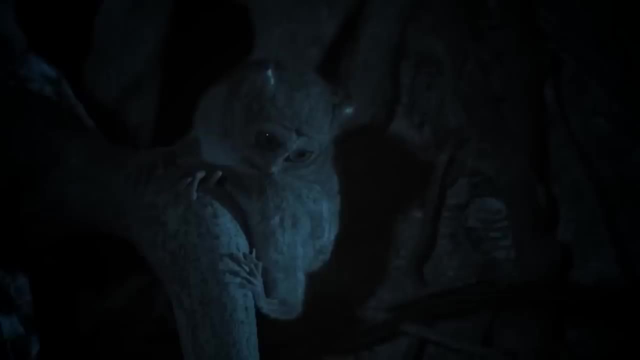 One of the smallest and rarest primates in the world had not been seen alive since 1921. It was thought to have died out, But in 2000, a group of scientists from Indonesia proved wrong, what people had thought for decades. The group was doing research in Indonesia's 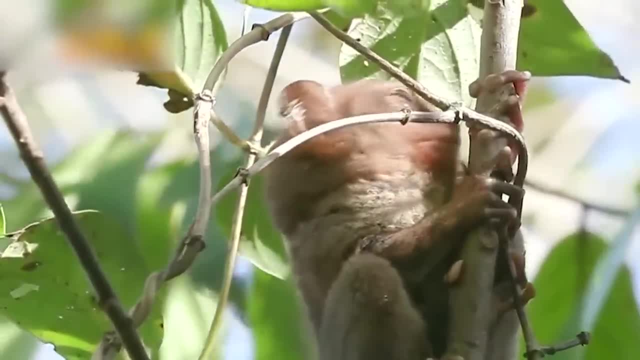 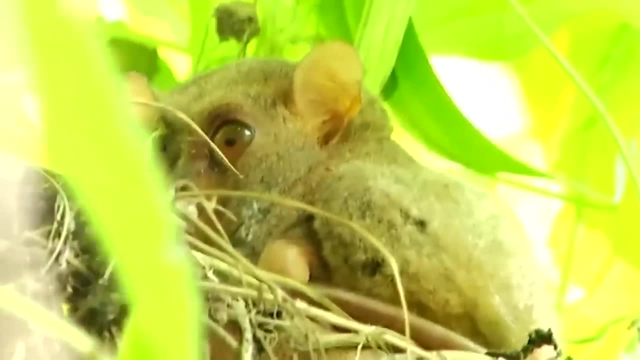 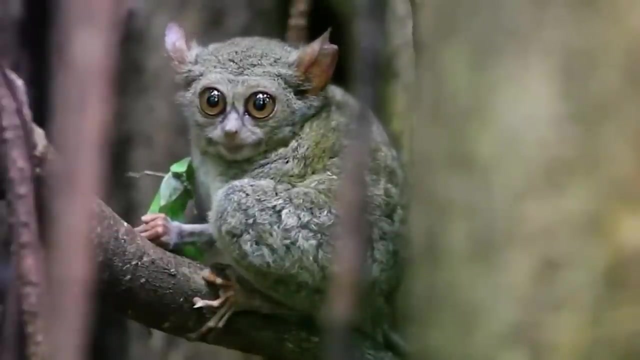 Sulawesi highlands, when they accidentally caught and killed a pig- 7. PIGMY TARSIER. Then later, a group of American scientists went to the 6,900-foot mountaintops of Lor Lindu National Park and caught three more tarsiers, Two males and one female. These were the first live tarsiers. 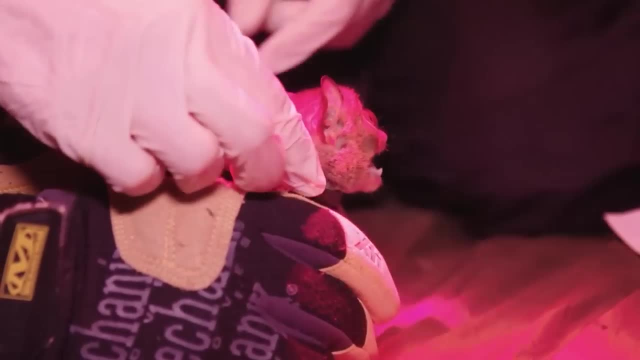 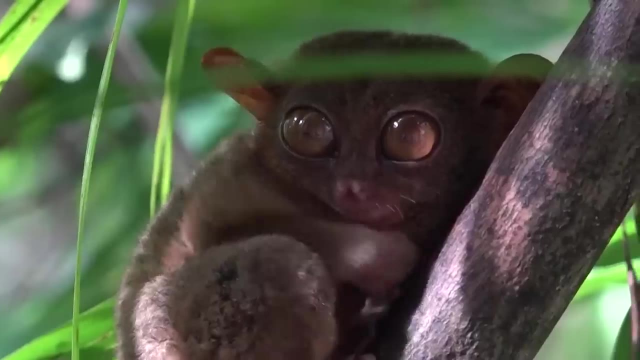 seen in 87 years. They put radio collars around the necks of the animals so they could track where they went. People have often said that tarsiers look a lot like Gizmo from the movie Gremlins. They're about the size of mice and they weigh only 2 ounces. They have small claws and big eyes. in. 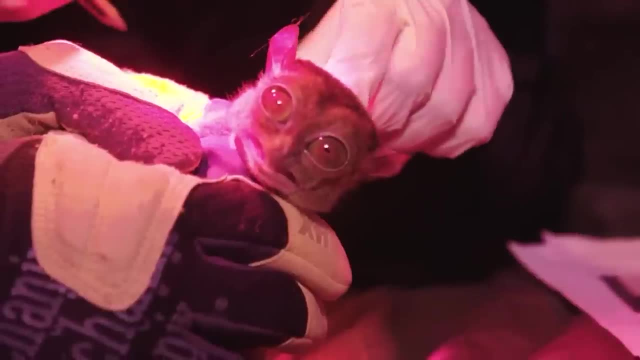 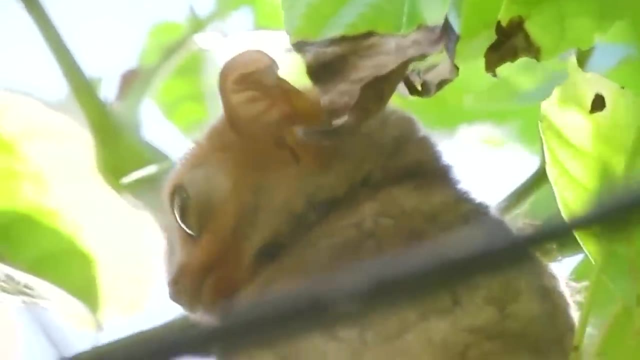 ears. They can turn their heads 180 degrees and scientists learned the hard way that they will bite if they think someone's a threat. Just don't give them water after midnight, or it might be you who ends up extinct. 6. BRUSHTALE POSSUMS. 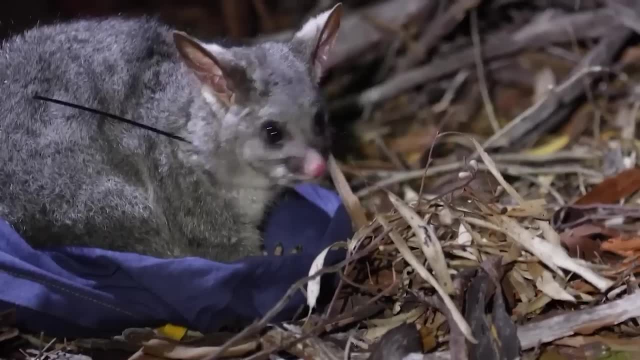 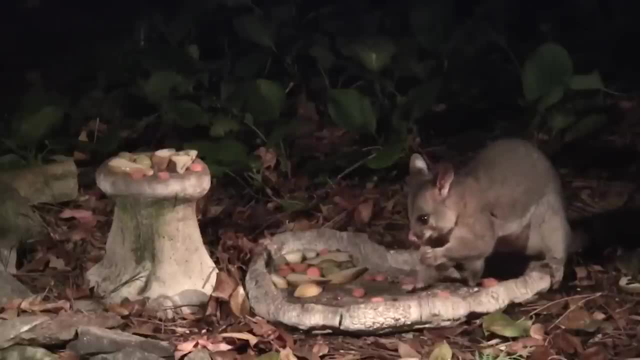 The scaly-tailed possum is one of the least well-known and most mysterious animals in Australia. New research shows that the so-called isolated East and West Kimberley populations are not that different from each other. They're not the same species, but they're not the same species. 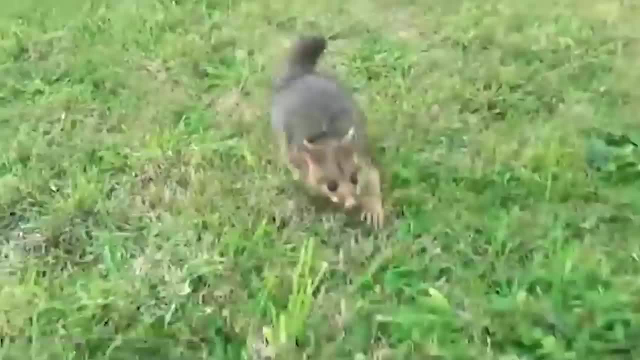 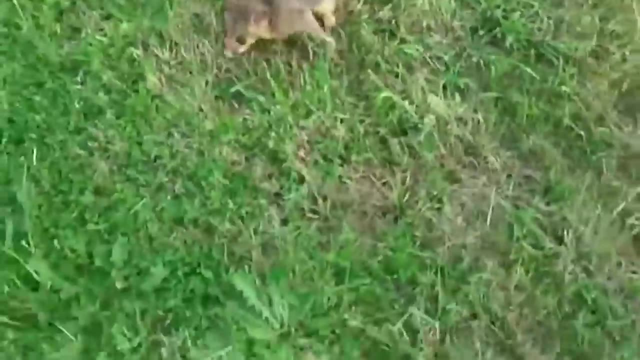 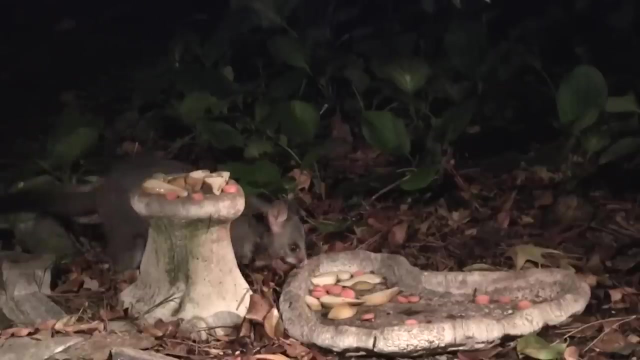 This means there are, or at least were recently, populations in between that haven't been found. Managing the species will depend on how this problem is solved. Where are the missing link? possums hiding? The possum with the scaly tail is a weird critter. It doesn't have any close. 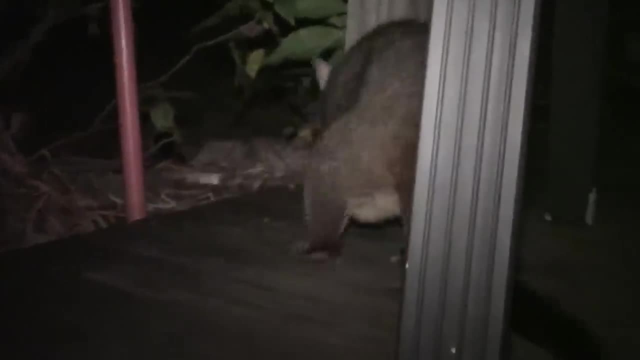 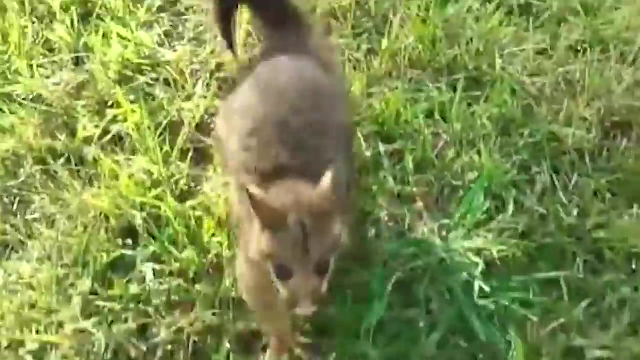 relatives, but the well-known brush-tailed possums of Australia and the Caucasus of New Guinea are related in a distant way. Unlike its distant relatives, the scaly-tailed possum needs rocky outcrops to hide in during the day. At night it comes out to eat in the forest around. 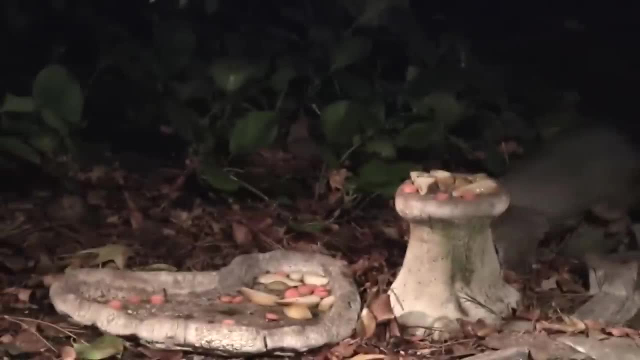 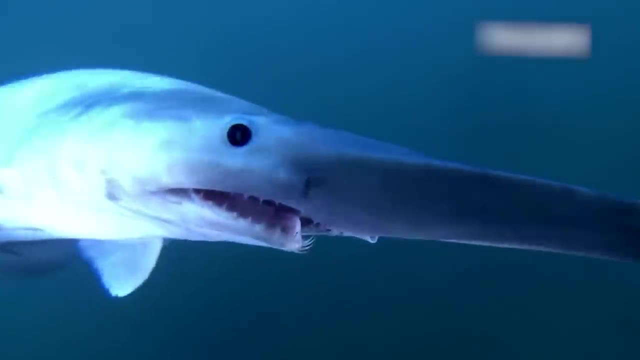 it. Possums have a strangely flattened head and most of the fur on their prehensile tail is gone. 5. GOBLIN SHARK, This Georgia shrimp captain, said it was the rarest and ugliest catch he had ever made. 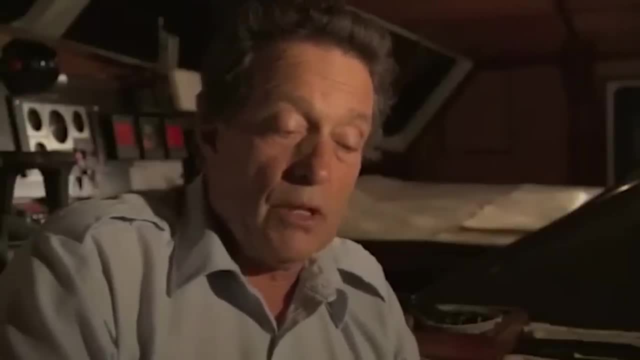 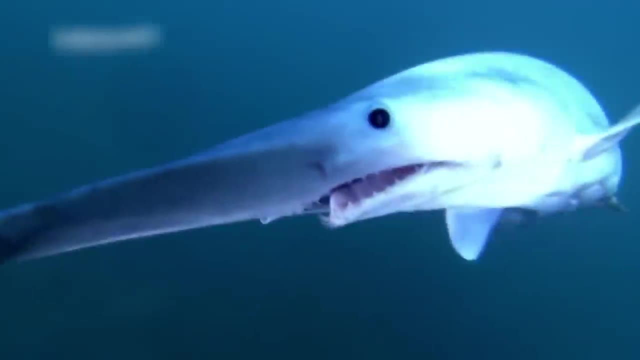 Captain Carl Moore was working about 10 miles off the coast of Key West Florida. He threw his net into the Gulf of Mexico and found a huge scary fish called a goblin shark. The goblin shark is a very large shark. Ocean researchers last saw this type of deep-sea shark. 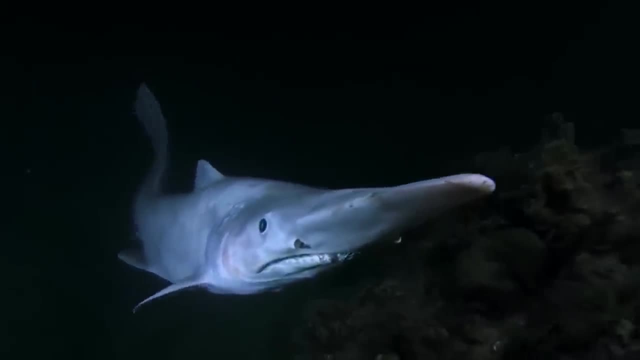 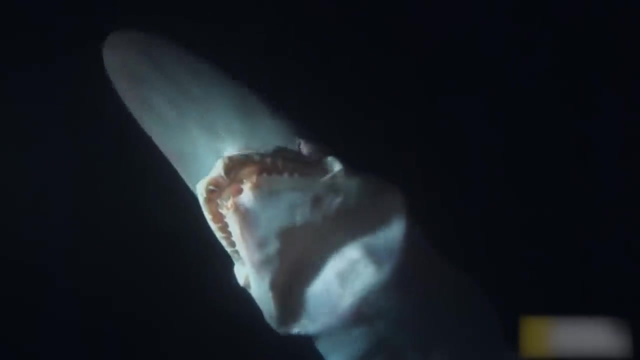 in the year 2000.. Goblins can be recognized by their long, flat noses that stick out from the top of their heads. When they open their mouths they show razor-sharp teeth, like the aliens in the science fiction movie Alien. Goblin sharks have been seen in the Pacific near the coasts of Japan. 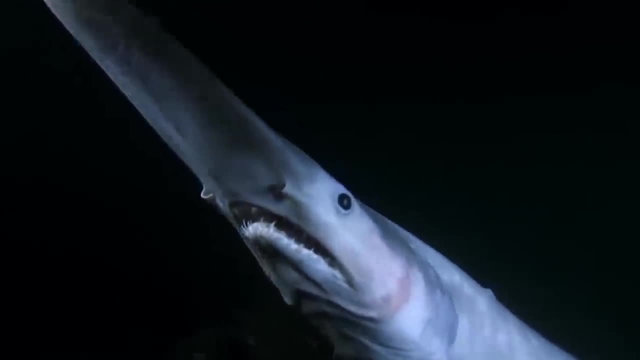 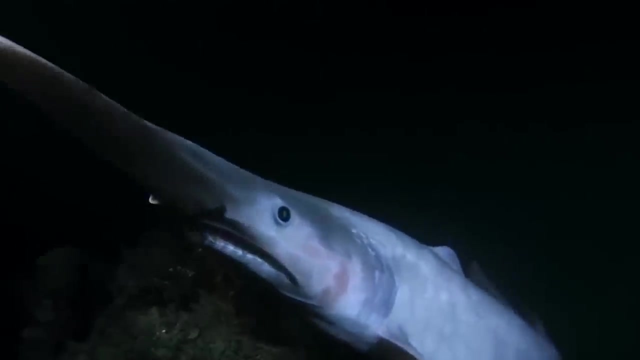 and California and as deep as 5,000 feet below the surface. Researchers were surprised by the most recent sighting, though. They can be as long as 10 to 13 feet, But Captain Moore's goblin shark was 18 feet long. He said that after taking pictures of the shark, he quickly put it back in. 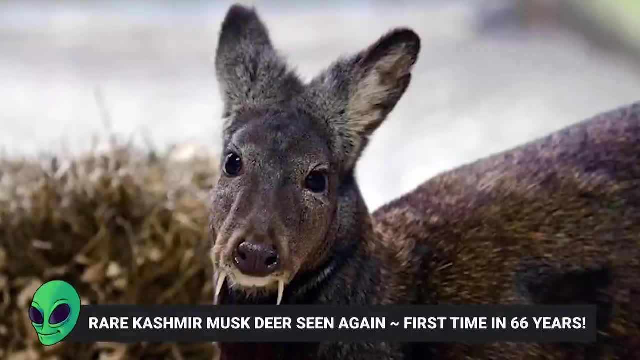 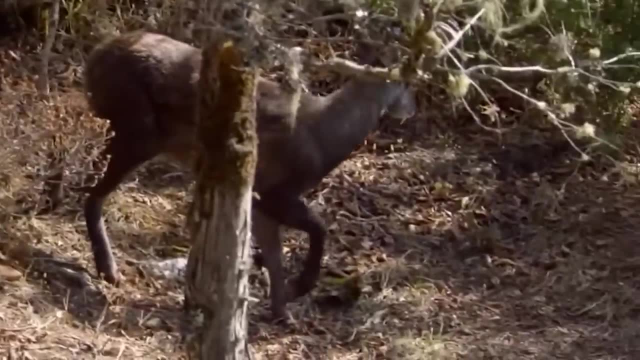 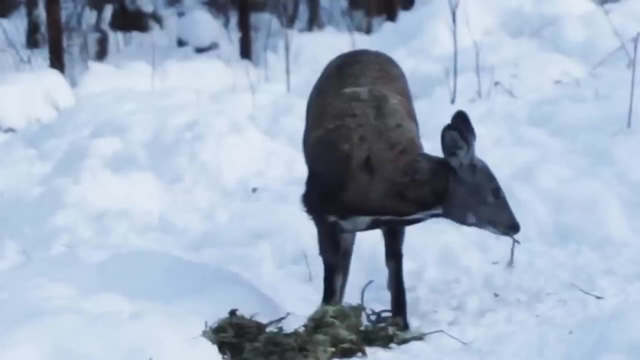 the water. 4. RARE KASHMIR MUSK DEER SEEN AGAIN FOR THE FIRST TIME IN 66 YEARS. The Kashmir musk deer, a small animal with horrifying fangs that look like vampire teeth, can still be found in the east forests of Afghanistan more than 60 years after it. 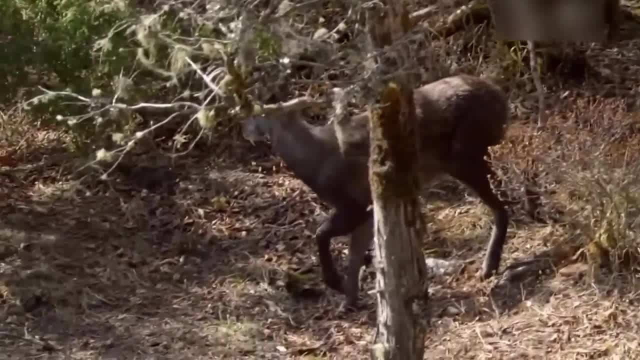 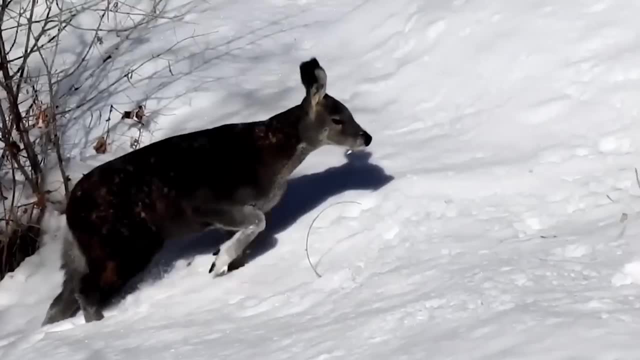 was last seen there. These Dracula-loving deer live in the Himalayas, central and southern Asia and Siberia. They like to live in forests and they tend to stay in the same area. They can run quickly up and down the steepest hills and are very sure-footed on the rocks. 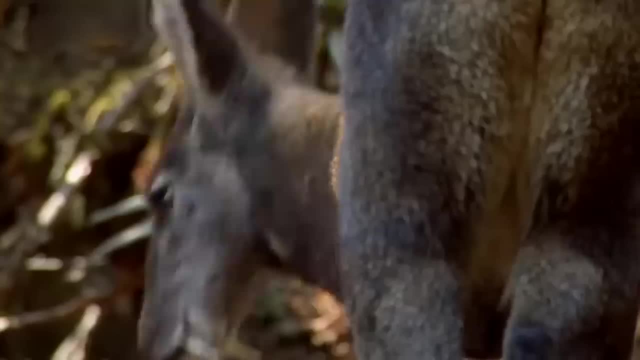 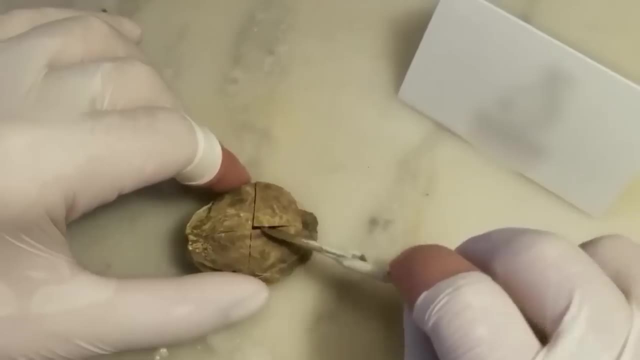 During the mating season, the male uses his unique tusks, which look like swords, to fight with the other males. People often hunt them for their meat or for their musk glands. On the international market, a kilogram of musk can sell for $45,000 because it's thought to have 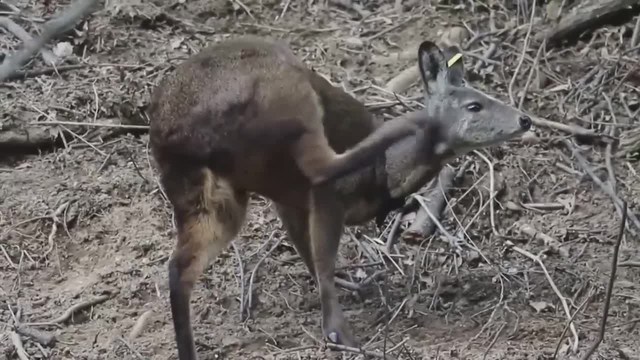 uses in cosmetics and medicine, Even though the musk deer are considered to be the most dangerous animals in the world. they are considered to be the most dangerous animals in the world Even though the musk can be taken from animals that are still alive. most musk gatherers kill the animals to get. 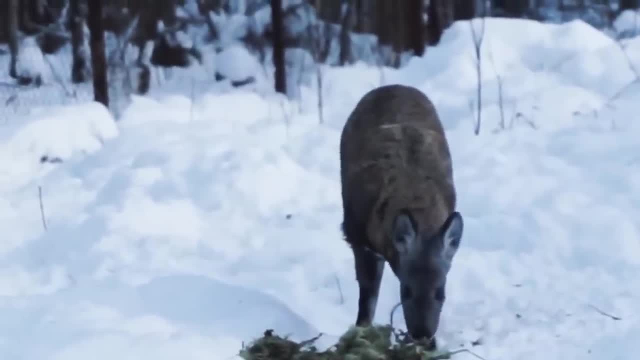 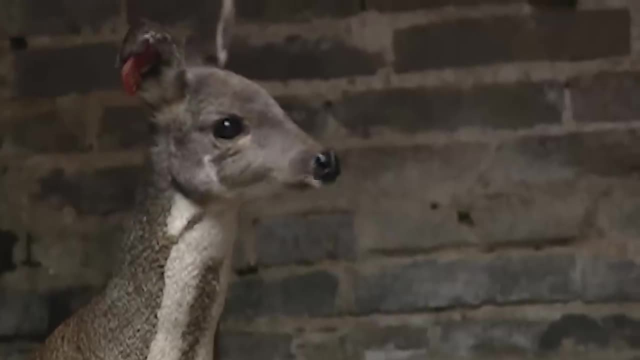 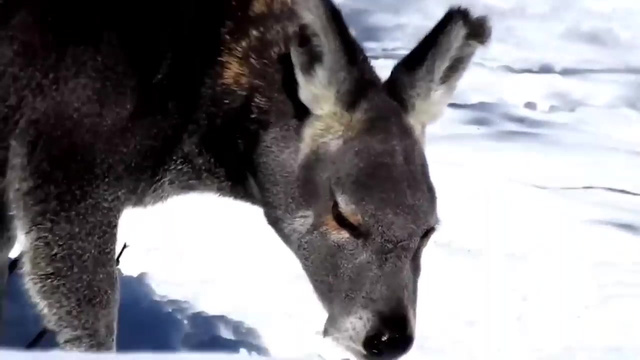 the whole sack. In Afghanistan, Nut Paludan, a member of the Third Danish Expedition to Central Asia, saw this species for the first time in 1948.. Three times they saw a single male in the same area. one time they saw a female with a young one and once they saw a female by herself, which may 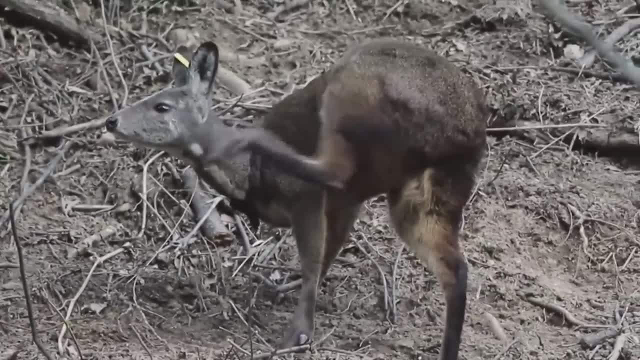 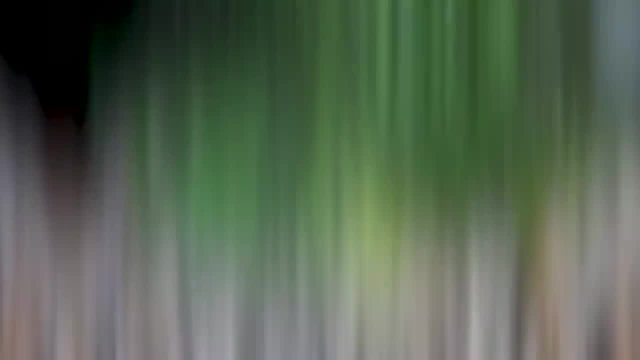 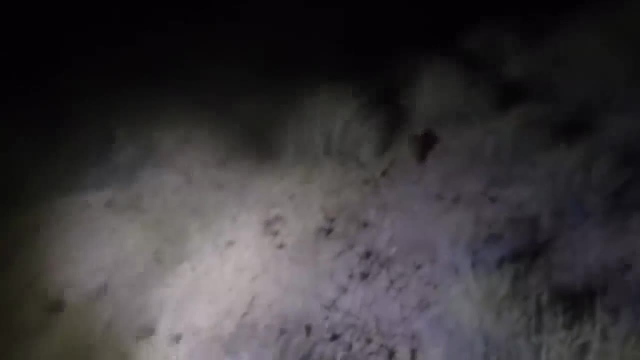 have been the same female without her young. That was until recently when this amazing and strange animal was finally spotted again. 3. Night Parrot. A few brief but unconfirmed reports from its former range and the discovery of two dead birds in Queensland in 1990 and 2006 only added to the mystery of the bird In Western Queensland in 2013,. 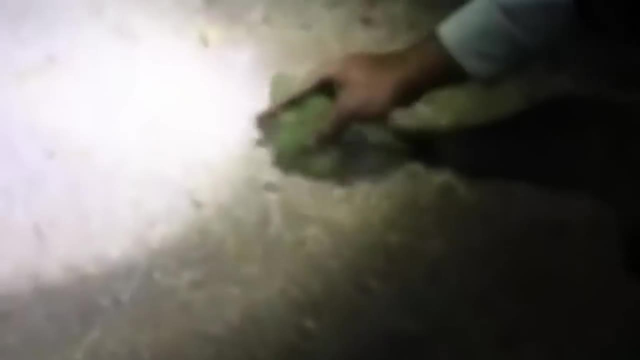 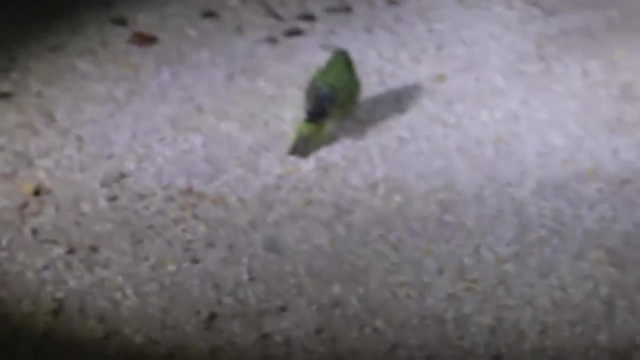 naturalist and wildlife photographer, John Young, took several photos and a few seconds of video of a real living night parrot, and the world was amazed. Seems like this beautiful bird was brought back to life. John spent many years looking for a night parrot, which is often called the holy grail. 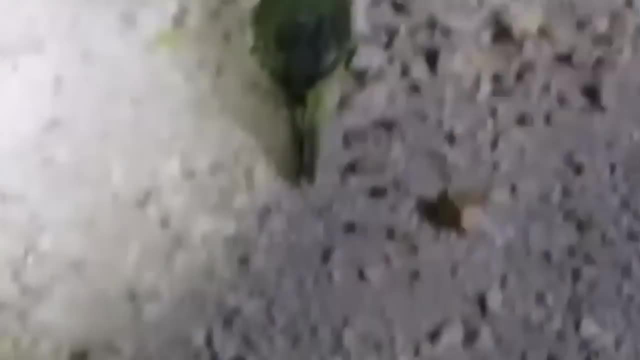 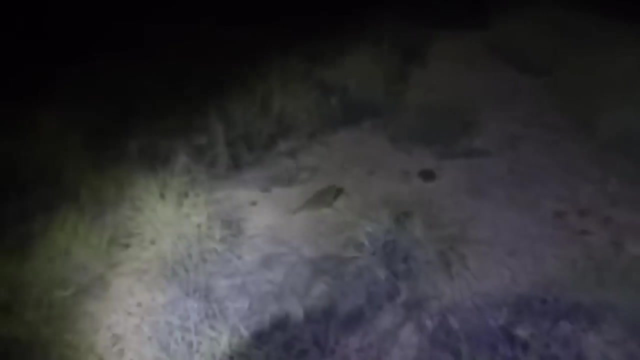 of bird watchers and naturalists, but he finally found one and got to see it up close. The discovery got so much attention around the world that the exact location of the only known populations of birds was kept secret to keep the birds from being disturbed. This kind of second chance does not come. 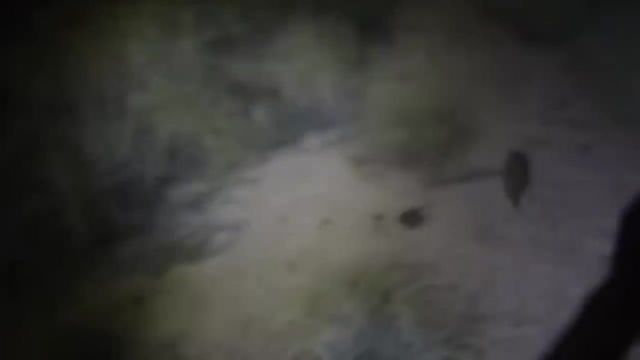 along super often. An organization called Bush Heritage has taken the lead to make sure that we don't lose this hard-to-find bird again. 4. Bush Heritage. The key to protecting the bush heritage is to keep the birds safe. The key to protecting 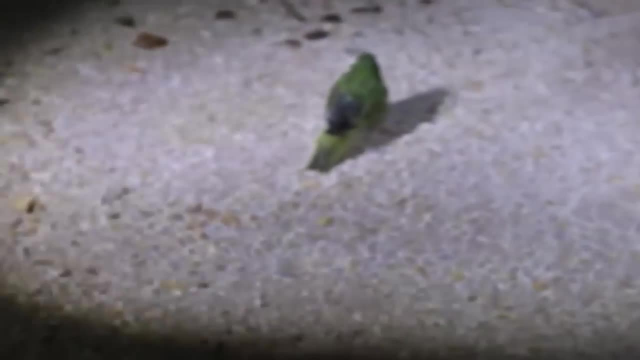 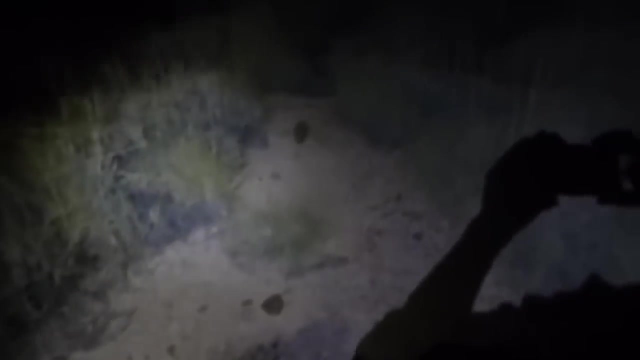 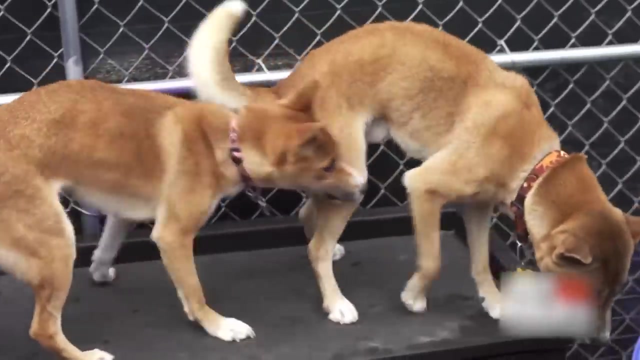 the bird is its habitat. Since they've been there for a long time, it seems like it's a good place for them, but we know they're in real danger, mostly from humans and invasive species. 2. New Guinea Singing Dog: The DNA of three wild dogs that were.